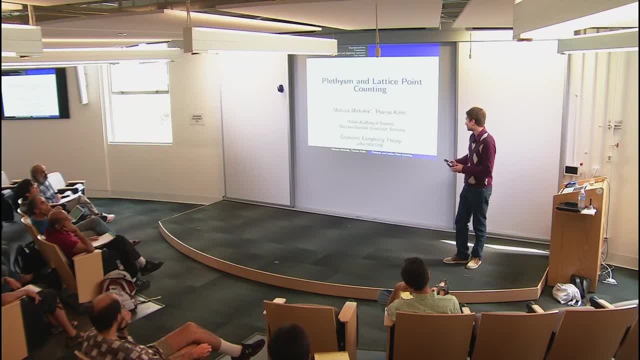 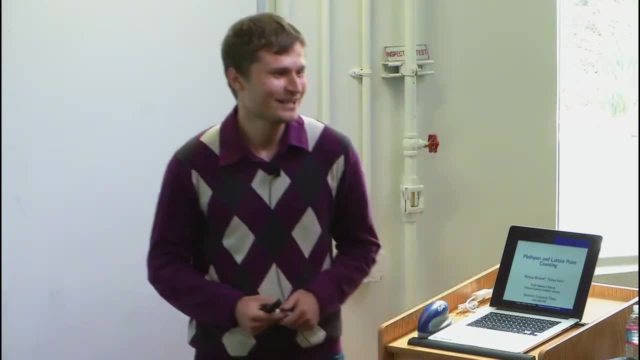 of previous talks and remove the intersection. However, I was not able to do it with the talk that just took place an hour ago, So I'm very sorry for the repetitions that will be present. I will be giving a very easy talk on a very classical problem: plethysm. 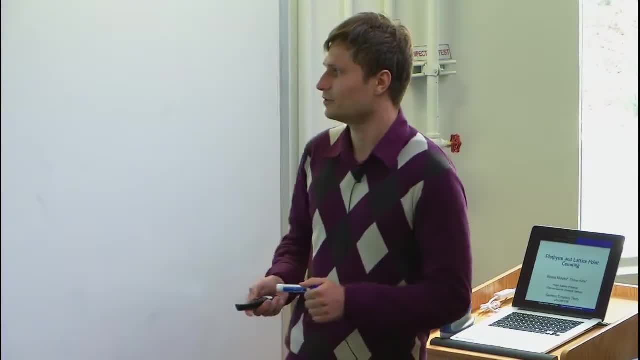 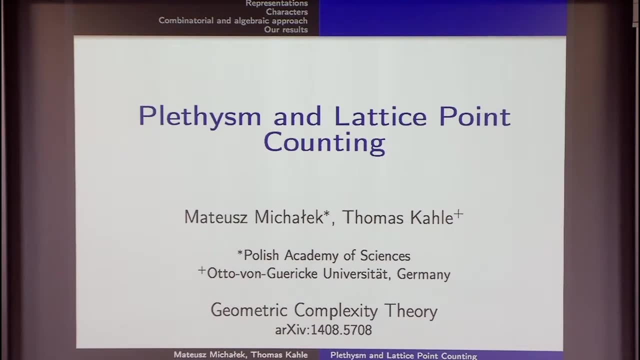 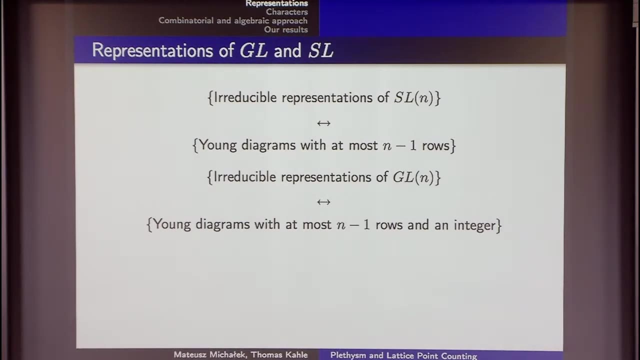 This is a part of a joint work with Thomas Kalle from Magdeburg, currently at Magdeburg. Please, if you have any questions, feel free to ask. So to show you how easy my talk is, I will start by reminding that irreducible representations correspond to young diagrams. 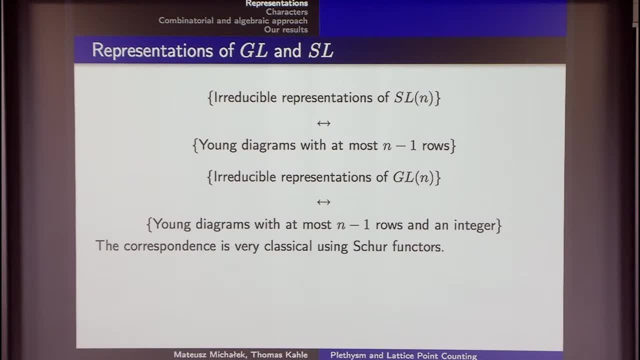 And I will even say more how one can think about it. Namely, I would like to think about it in terms of sure factors. So to a young diagram I associate a sure factor. How does it work? I take the space V if I consider the group. 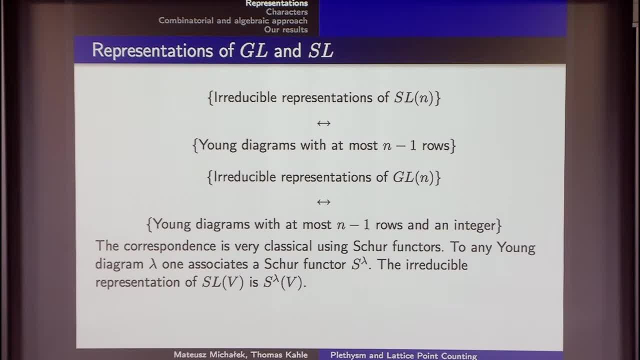 SLV. I tensor it as many times as my young diagram has, as many boxes as my young diagram has, And then I act on the tensor. I take the power with the young symmetriser. So most of you know young symmetrisers Here. 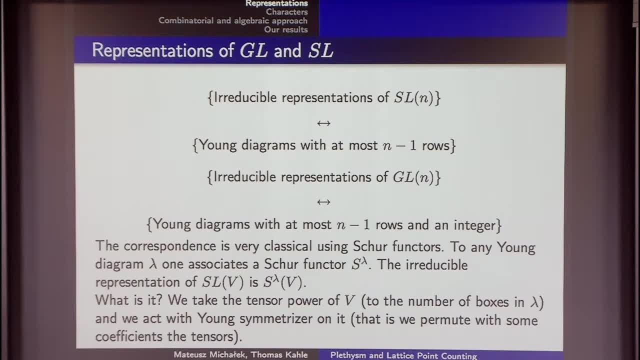 you can consider them just as a map that takes a tensor, permutes it and associates certain coefficient and sums up. So, for example, for the symmetric power, you just take all possible permutations with coefficient one, And for the wedge power, you just take also all possible. 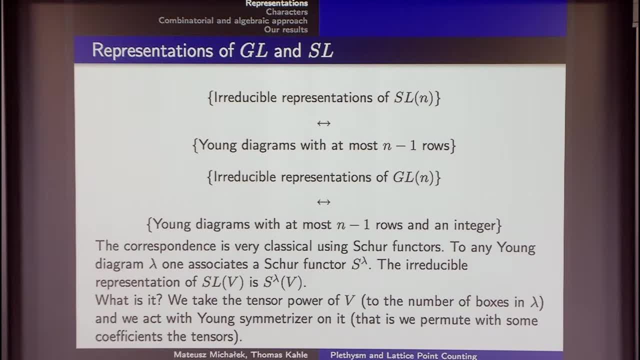 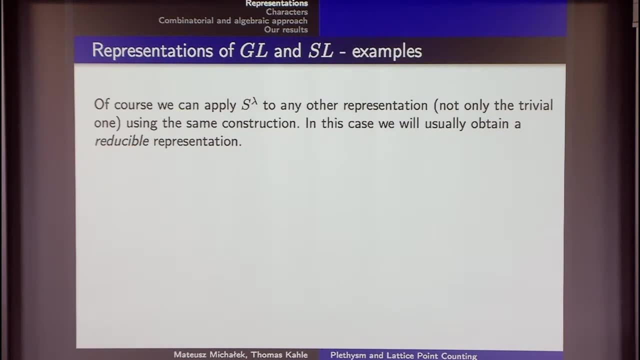 permutations, but the coefficient is equal to the sign of permutation. So, as we know, like this we can get all irreducible representations of SLV, varying just the young diagram. But as we defined it it really didn't matter that the starting representation was the most. 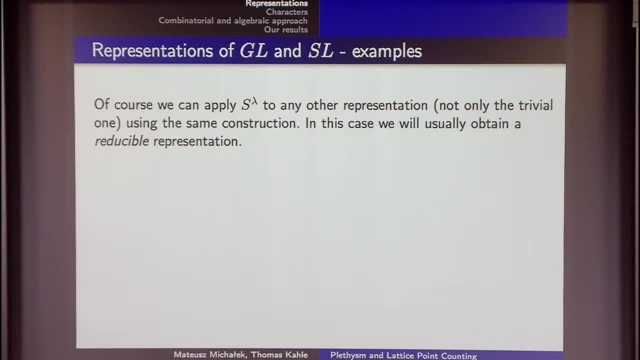 trivial one, V. I could have done it for any representation. Take the tensor power act with young symmetriser. So in fact S lambda is a factor from representations to representations, If I apply it to the trivial, just to V. 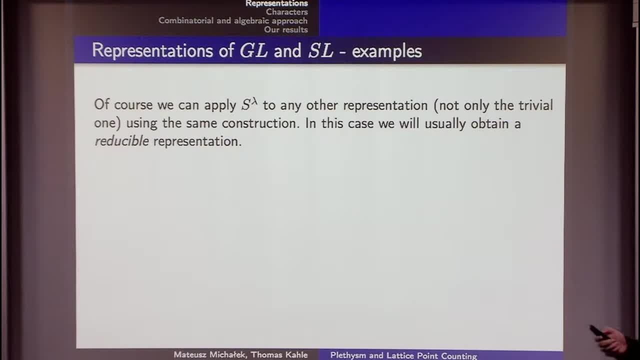 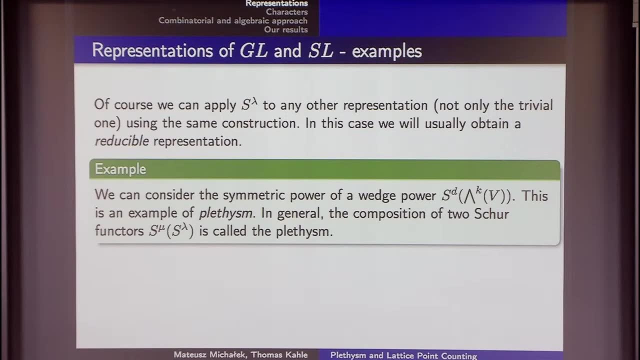 then I get the irreducible representations. But when I start applying it to other, more complicated representations, in general I get reducible representations, And this is what I call the platism, So application of a sure factor to another sure factor. So 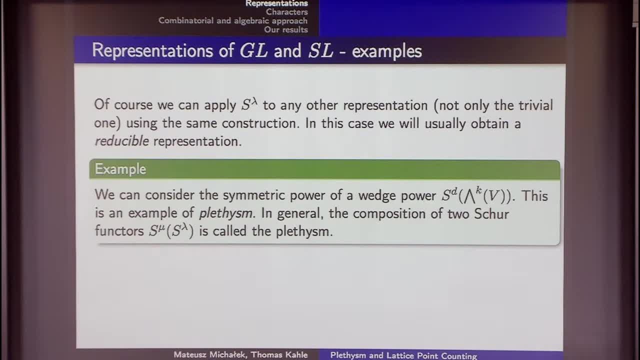 here I stopped omitting the vector space V, as I usually will not do So. I get the irreducible representations V, but when I start applying this to a pre domain, then I get the Y inverse vector space, which is the non-dḍ. X as the N vierge vector will not be interested in it. As long as V is sufficiently many-dimensional, the decomposition of such a composition in terms of the young diagrams is just the same. So the most well-known sure factor is for sure the symmetric and the wedge power. And 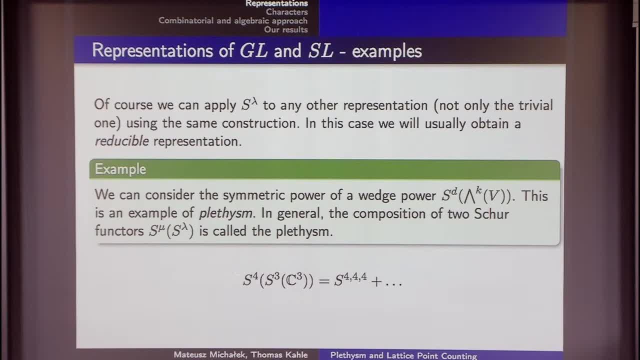 and also in this talk. these are the two sure factors will be mostly interested in. So here is an example. We take s4 of s1, and so in the example we have S4, and and and, so the integration. on the S4 of s2, we take S1, and S1, and S2, and S2, and S2, and so on until we get the 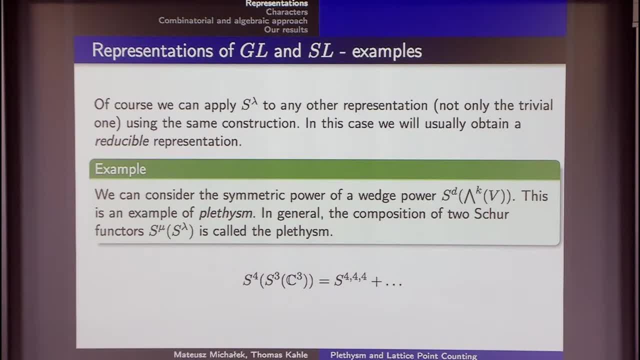 of s3 in c3, and when we decompose it, such thing with multiplicity 1 appears. So here I mean a Young diagram with three rows and four boxes in each row. So the first question is: what is it and when did it appear on this conference? 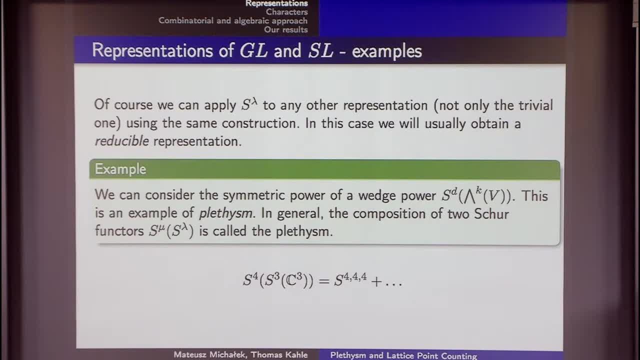 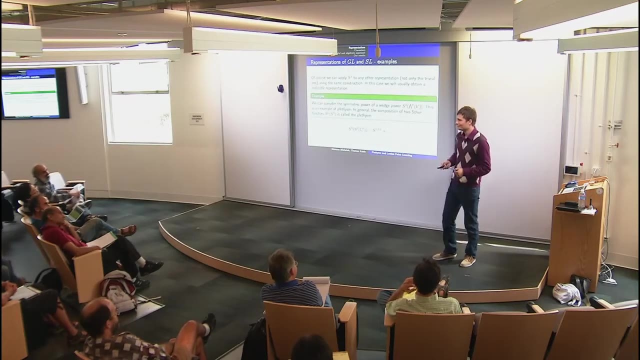 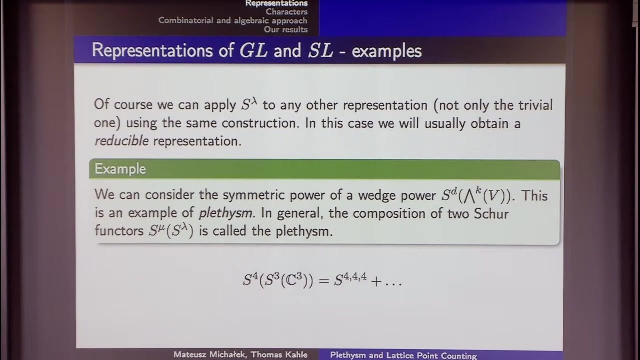 Yes, I mean on Monday we saw the degree for invariant for plane cubics, Great. So Bernsturm gave a very nice talk about invariants and we see that if we know Plattism in particular, invariants Appear there and we can recognize them as rectangular shapes. 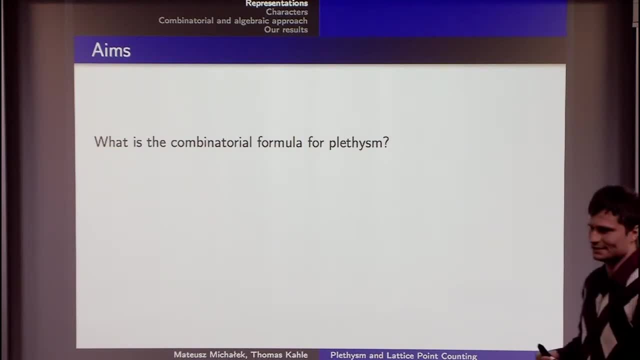 Great. So I hope this is like one of the motivations to understand Plattisms. So if we just focus on symmetric powers of symmetric powers, it means that we are trying to understand polynomials in coefficients of polynomials. So unfortunately, I'm sure. 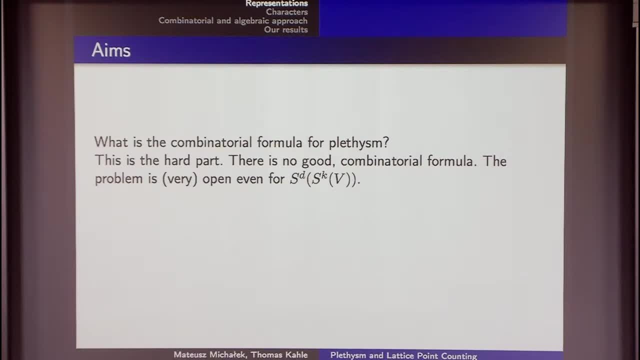 The idea is that almost every expert in a representation theory has got his own favorite way to compute the Plattisms, but there is no really good combinatorial formula And also many, many speakers refer to it. There are many formulas how to compute it, but I guess that we are still looking for. 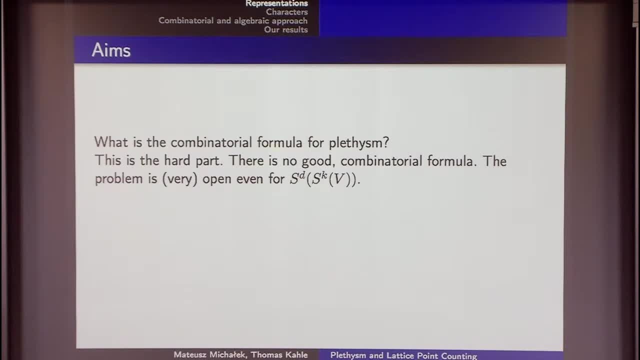 a really good, really fast one, even for symmetric powers. So the aim, The general aim, would be to fully understand polynomials in coefficients of polynomials. So here this will be like degree D polynomials in coefficients of degree K polynomials. 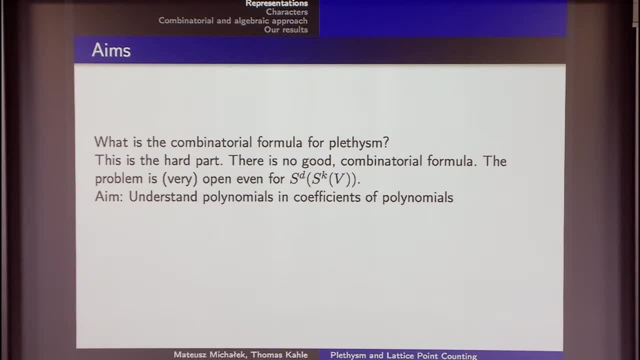 But we already know this is difficult. This is very, very difficult. So the aim of the talk will be a little bit different, a little bit more modest. So understand low-degree polynomials in coefficients of arbitrary polynomials. So I would like to make it very clear. 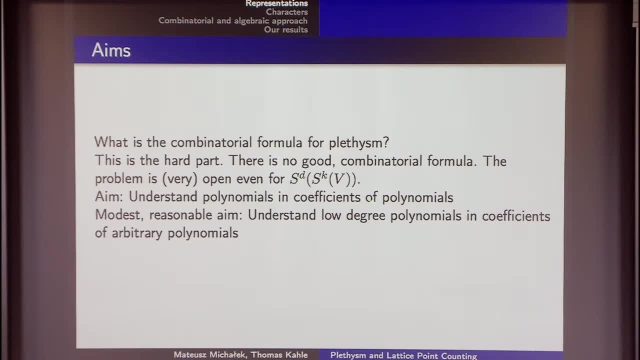 I will be considering small d and arbitrary K. Yes, Any questions at this point? This is my aim. I don't care about complexity, about other things. I really want to understand low-degree polynomials in terms for arbitrary inner polynomials. 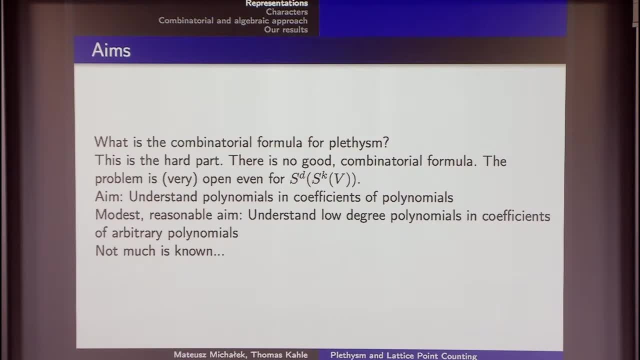 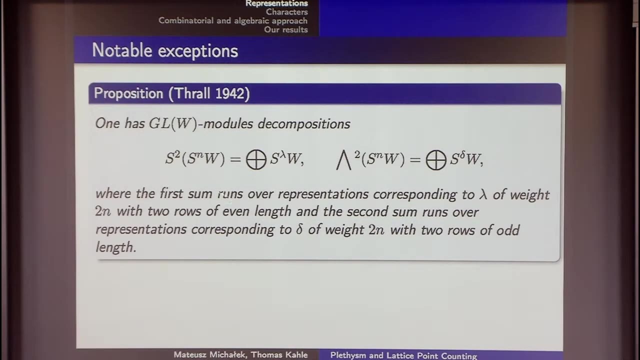 And you might be disappointed. Not much is known about this, Even for For small ds. But not much doesn't mean nothing. So what is known? So one of the first results is due to Thrall in 1942. He provided a formula for the second symmetric power of nth symmetric power. 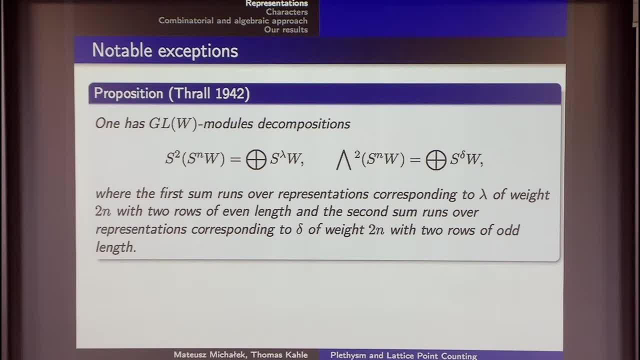 And it turns out that the multiplicity is always 1 or 0. And it's precisely 1 when your lambda has just two rows and both of them are even So for me. I would interpret these results that Thrall understood: quadrics in coefficients of arbitrary polynomials. 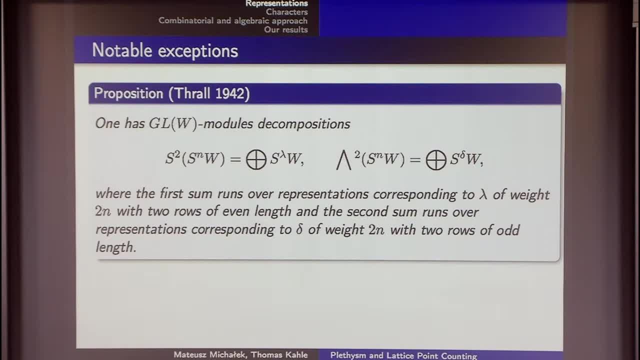 And you already can see that- an important thing that was often referred to during this conference- that the lattice structure plays a role. So it's not only inequalities or polynomials, but the rest. modulo some number gives you the result, whether the multiplicity is 0 or not. 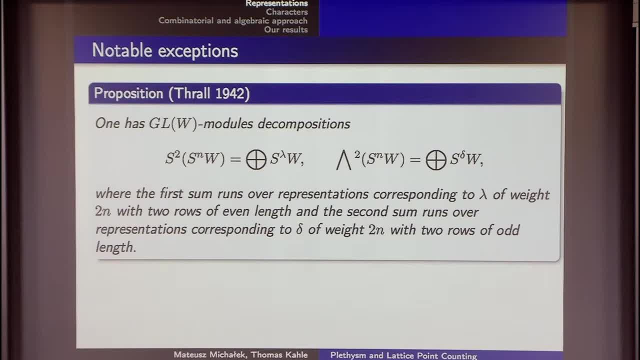 Here it's very easy, just modulo 2.. But later we'll see that such things are quite important. Okay, so we understand quadrics. And, of course, when we understand quadrics, what's the next natural question that people try to answer? 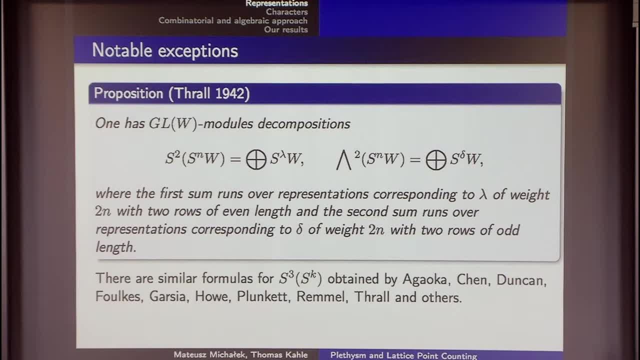 Cubics And cubics we also understand. So there are precise, explicit formulas to decompose S3 of S3.. This is not very, very difficult. There are many people who obtained So this already is later than 1942.. 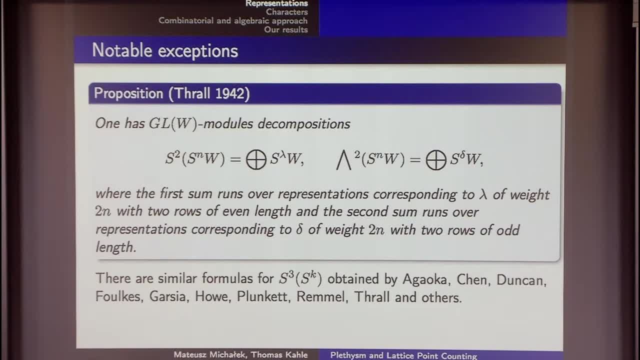 There are many different formulas, But in particular there are explicit formulas. I should say that also formulas for S, mu, S k- where mu is arbitrary partition of 3, are known Great. So what about quadrics? There is a paper of Howe where he says how he can obtain formulas for quadrics. 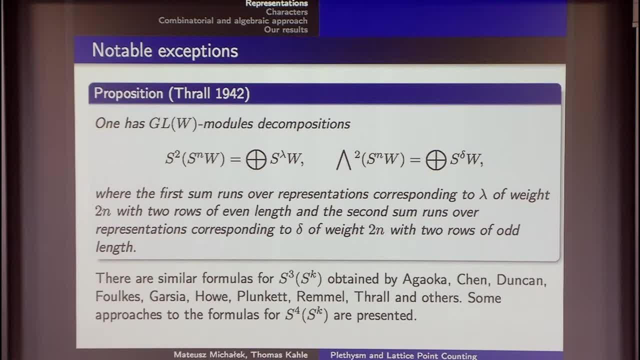 And he also says that interested people can contact him. but he will not put money that the formulas are correct. He just claims that his methods are correct to obtain the formulas. That's something. That's something At least we've got good methods to. 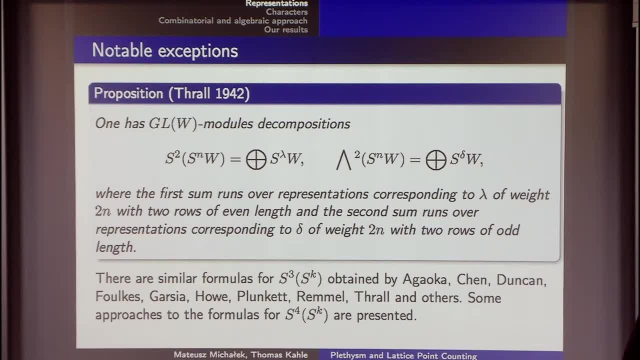 Yes, I did, Yes, I did, and he replied great. So let's say that quadrics can be understood. So what is the problem, you may ask? I mean, how can someone have methods but he's not claiming that the result he has is 100% correct? 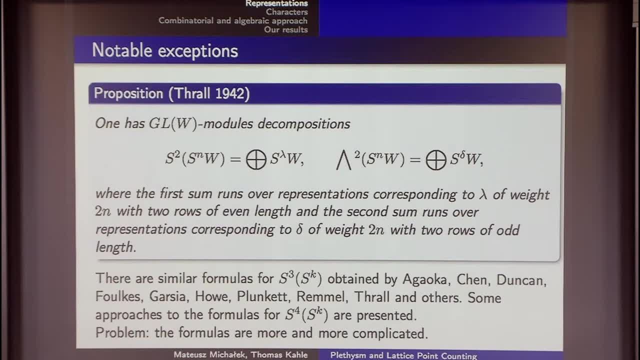 The thing is that this formula, the formulas are more and more complicated, And this I should say as for S k, I mean these are still quite old results, but many different approaches to S mu, S k when mu is a partition of 3,. 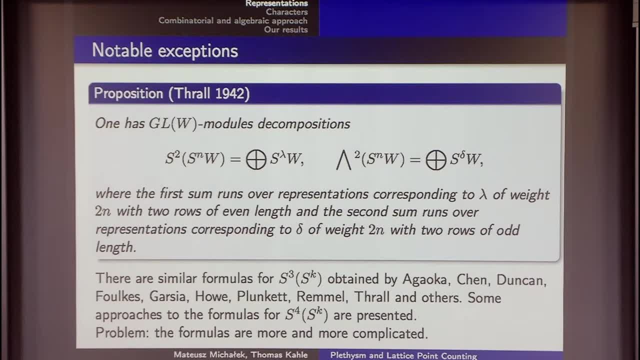 there are papers after 2000 about that Great. So the formulas of course become more and more complicated, But there are no negative signs there, right? I mean, okay, This is not a summation formula, This is an explicit formula. 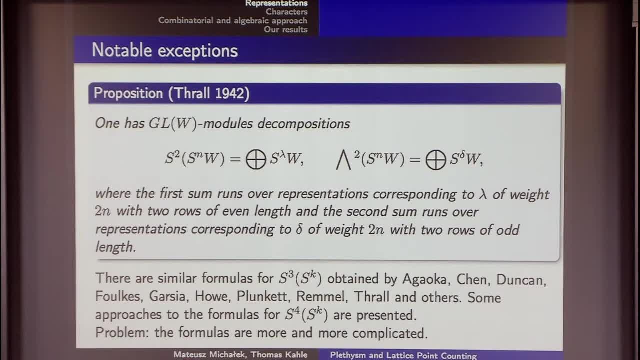 So it's a function in k and lambda an explicit function. So let's say you take the length of the second row, you add to it k, you divide by 2, you take the floor and this is the multiplicity. 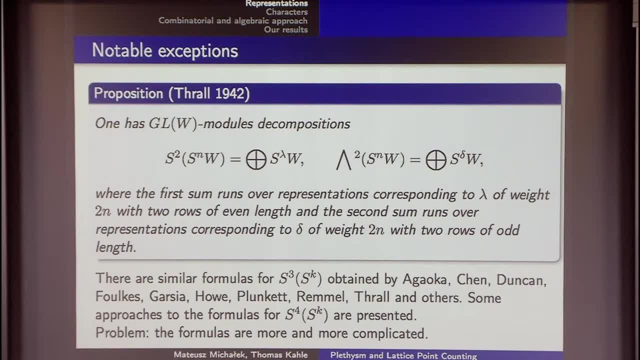 But do you subtract? is the question. Well, a polynomial has subtractions, But it's a formula. It's a formula, It's a really. But the question was: do you need to subtract? Yes, No, no, no. 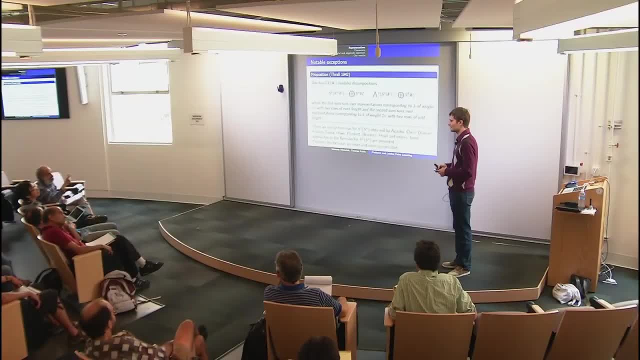 When you write down that thing like you wrote down, is it like that? Is it like that? So here the coefficient is like 0 or 1.. So this one I would interpret as a function that takes lambda 1 and returns 0 if lambda 1 is odd. 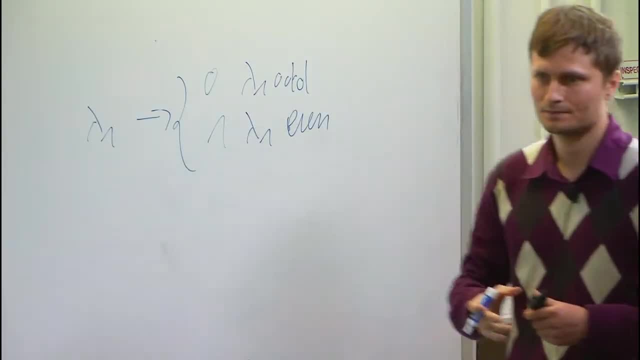 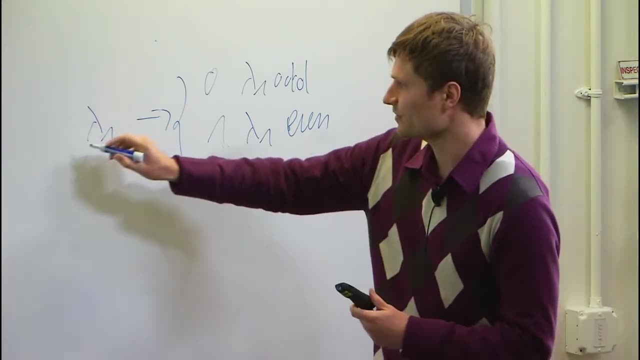 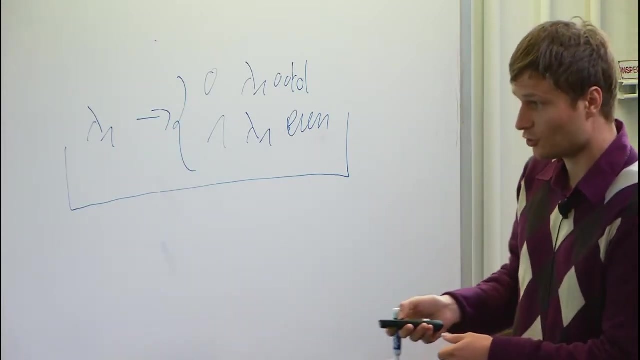 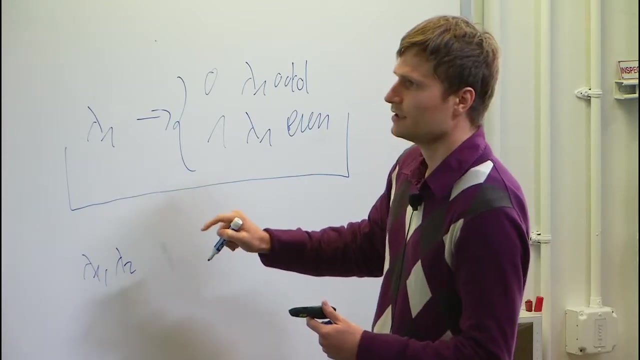 and 1. if lambda 1 is even This formula, I interpret it as such a function. And the formulas for S3 and S4, they are of such a type. They take, of course, more lambdas. They take, they take, yeah. 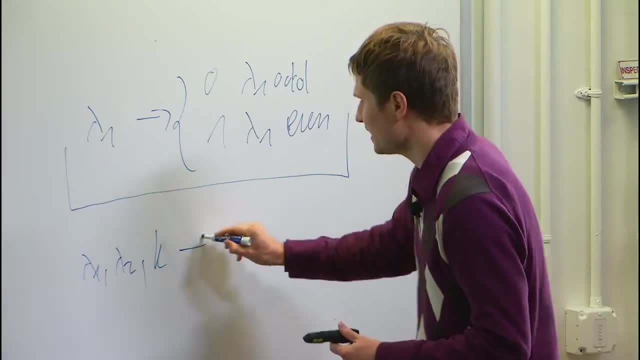 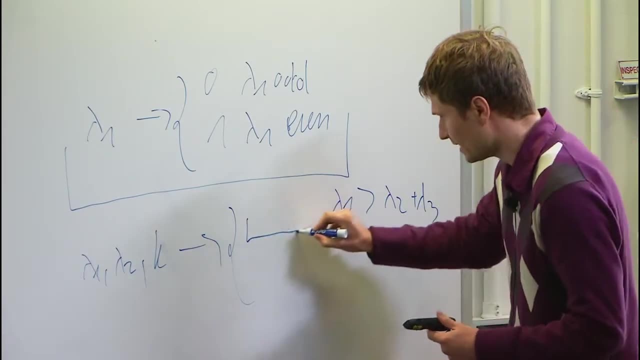 they take, they take, let's say, let's say k, And then it's like if lambda 1 is greater than lambda 2 plus lambda 3.. And here an explicit coefficient that can have minuses like lambda 1 minus lambda 2. 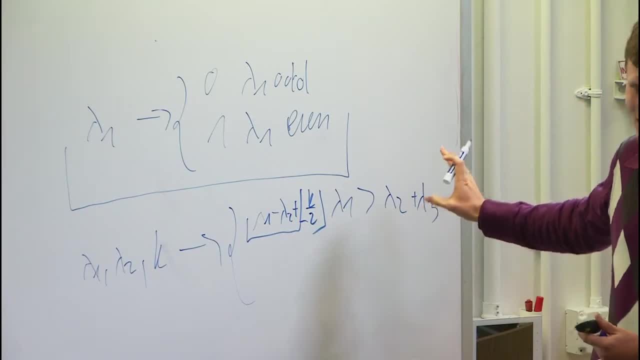 plus floor of k divided by 2.. I mean, this is not the result, but I'm just saying what type of formula one obtains So that formula can it become negative? No, yeah, I mean it's a formula for the multiplicity. 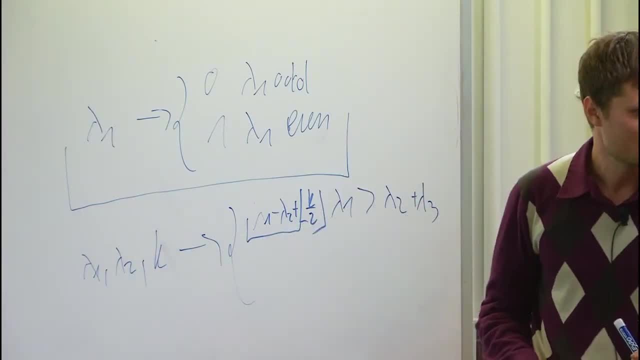 So when you evaluate it on the reasonable lambda and k, His question is: are there monomials in the formula that have a negative formula? Yes, Yes, I think that's the question. Yes, But we are not computing combinatorial objects of certain type. 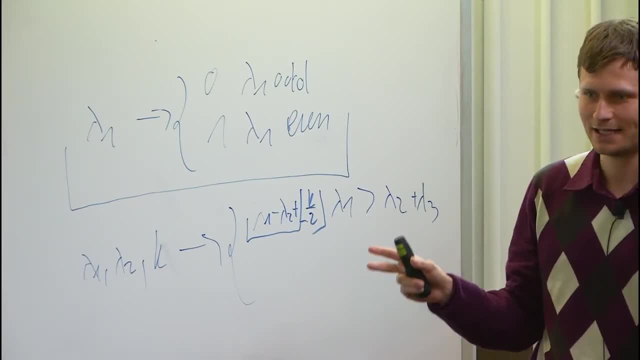 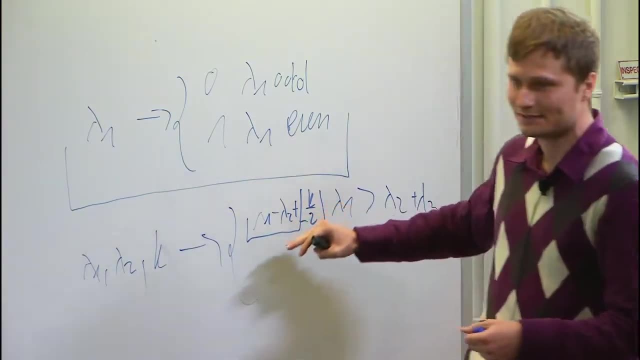 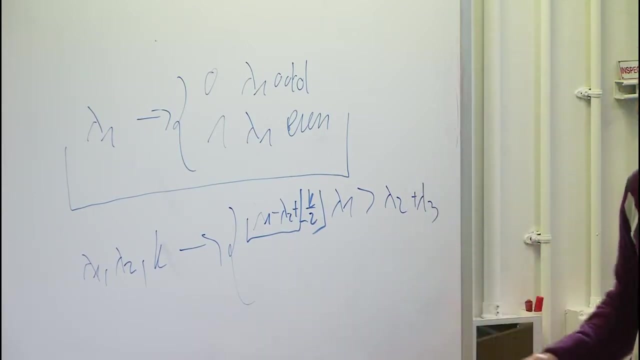 and subtracting them. So this is not like like the usual problem that happens that you compute certain types of combinatorial objects and you start subtracting them. It's an explicit formula: You are not computing any objects. Okay, so what would be the approach? 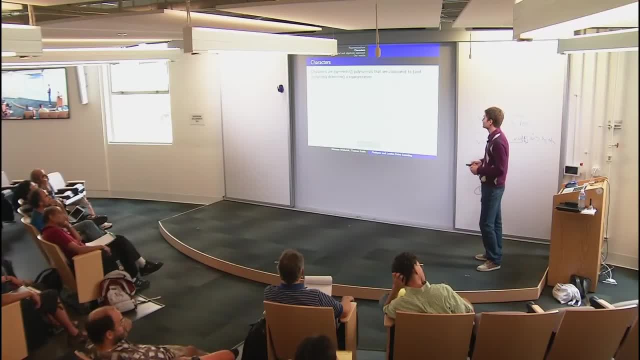 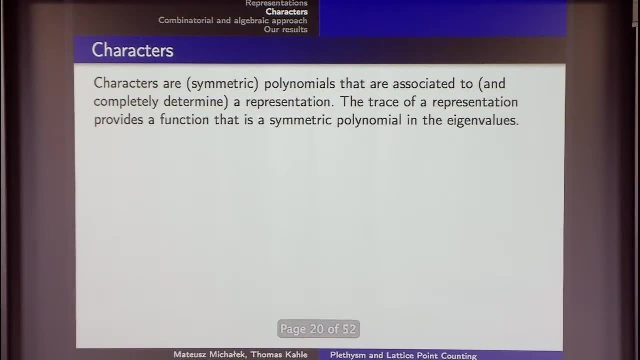 The approach is as usual and as presented on a previous talk, through characters. So you probably didn't forget in one hour that characters are symmetric polynomials associated to representations and that the trace of a representation is a symmetric polynomial in eigenvalues And for irreducible representations. 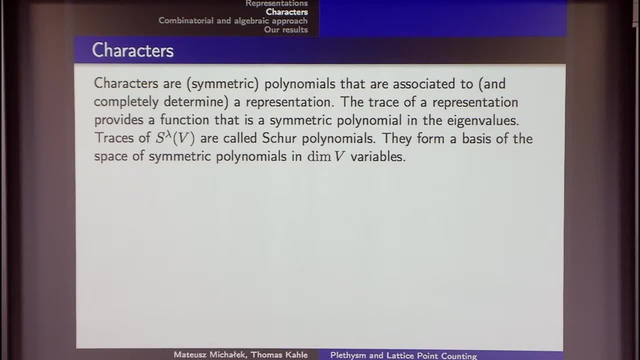 we've got super important functions that are called sure polynomials and form a basis of the space of symmetric polynomials. I even prepared an example, but I guess it's very clear by now that if you take just a two-dimensional vector space and if you act with 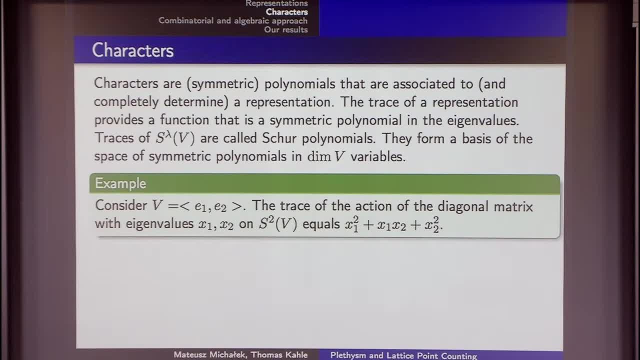 SL2, the character is like this: a complete symmetric polynomial. Yes, this one comes from the action on E1 times E1.. This one comes from the action on E1 times E2.. This one comes from an action on E2 times E2.. 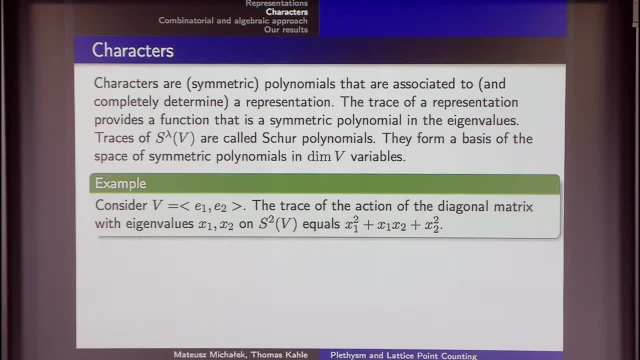 Yes, so this is a complete symmetric polynomial. You can easily see that for symmetric powers, you will always get a complete symmetric polynomial of this degree And I will denote it by H. So H, for me, will be a complete symmetric polynomial. Why are we interested in characters? 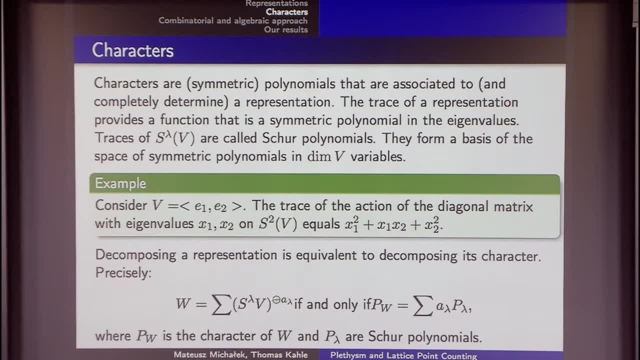 Because decomposing a representation into irreducible components is just the same as writing the character in terms of sure polynomials with coefficients, because they form a basis, everything is clear. So what is our aim now? Our aim now is, of course, 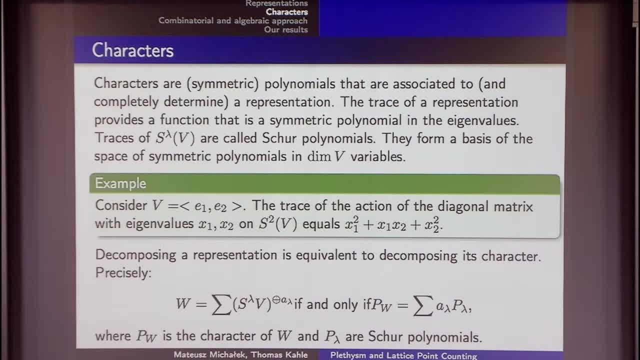 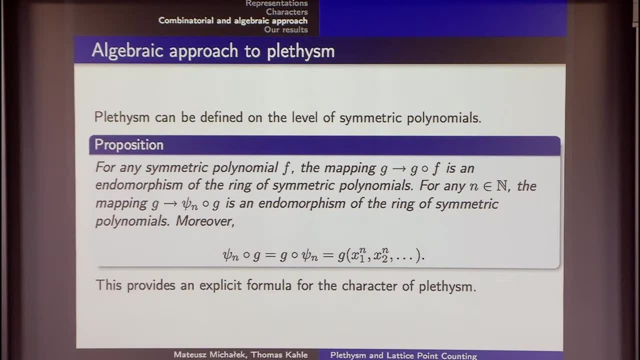 to understand the character of Pleiades And later to decompose it in terms of sure factors. So first we have to go from the Pleiades that was defined as composition of sure polynomials to the level of symmetric polynomials. So here the circle. 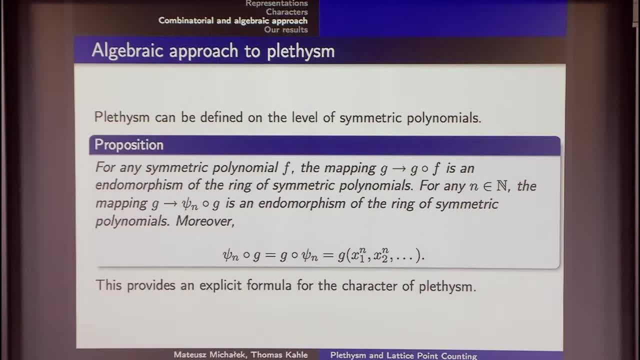 will be the Pleiades, And it turns out that, of course, you can do it on the level of symmetric polynomials. So if your G and F represent sure polynomials, then this circle will represent their Pleiades, the character of the Pleiades. 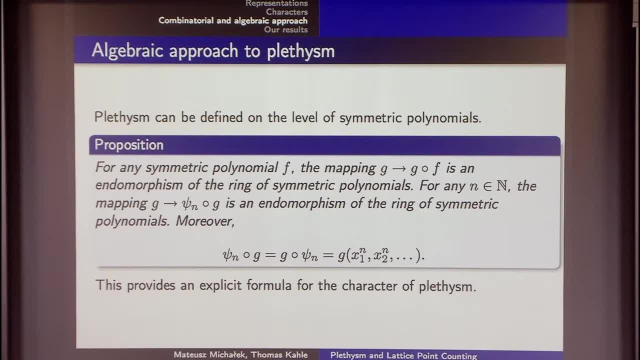 And this Pleiades has very easy and nice properties, namely in the outer thing it's an endomorphism of rings, of symmetric polynomials, And if the outer thing is just a power sum. so phi n is a definition, phi n of x. 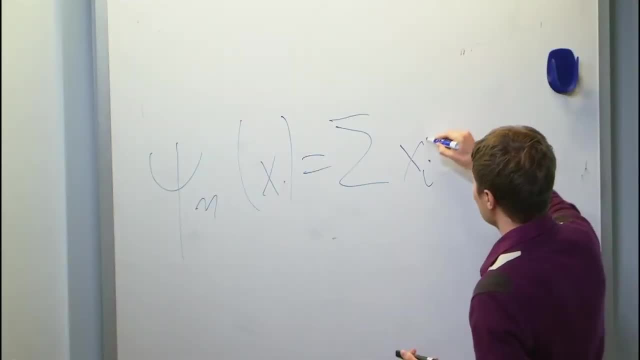 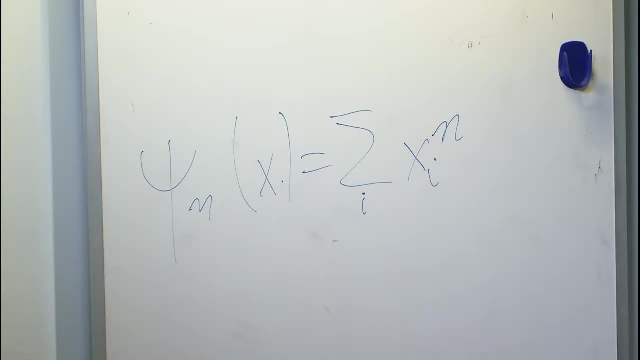 I just mean sum of xi to nth power. It will be a very important function for me. So if you do not like to compose sure factors, you can consider this as a definition of Pleiades on the level of symmetric functions, Because any symmetric function 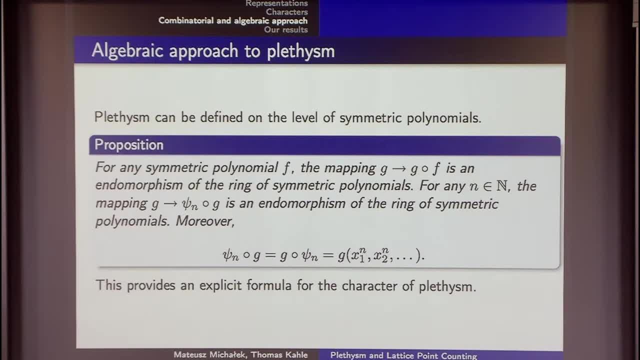 can be expressed in those phi's as a ring. generally, It's generated by those sorry, by those psi. And then, when you express your outer thing in terms of psi, using the fact that it's an endomorphism of rings of symmetric polynomials, 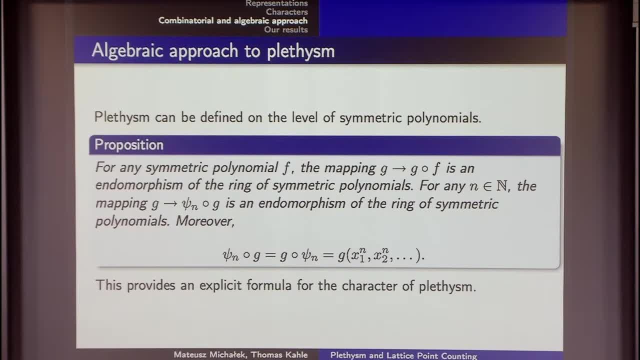 and applying this formula, you can compute arbitrary Pleiadisms. So some people are nodding, but I'm not sure. if it's clear, Most people are nodding, Yes, but they do. Yeah, well, that's They do. 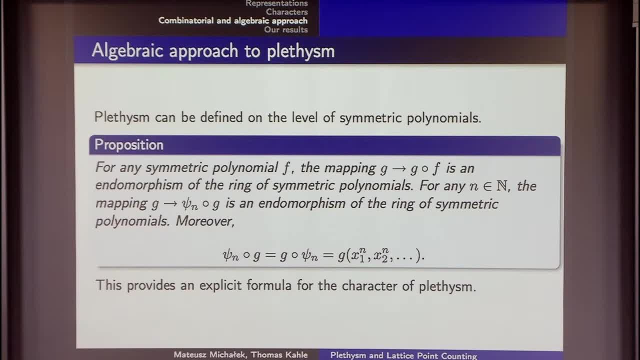 So, so, so so. so is it the case that you, just, you know, this is the point where you just plug in all the terms of xi into g. that's the general formula: Yes, yes, yes, here you see, yes. 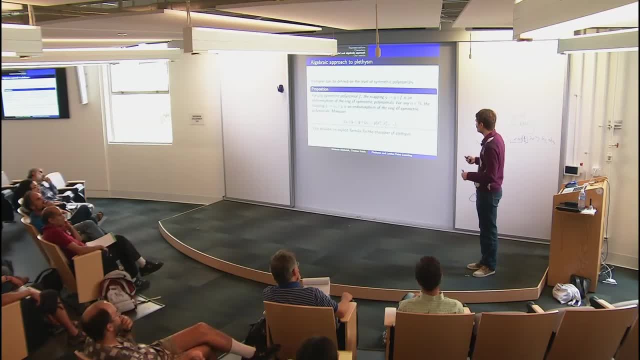 But that's the general formula for Pleiades: Yes, but, but, but. but I mean I prefer to do it this way because for, for for further application. So right now we will just use this proposition. If you would like to know more, 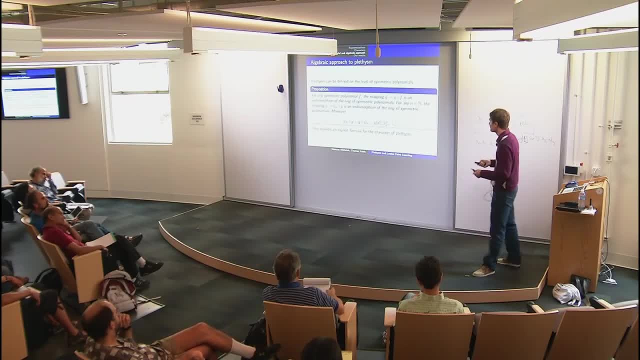 I mean, this is like in McDonald's book, very classical, So let let's do it for Pleiades. So I repeat the strategy: Express the outer thing in psi's and then use the fact that this is the endomorphism of ring of symmetric polynomials. 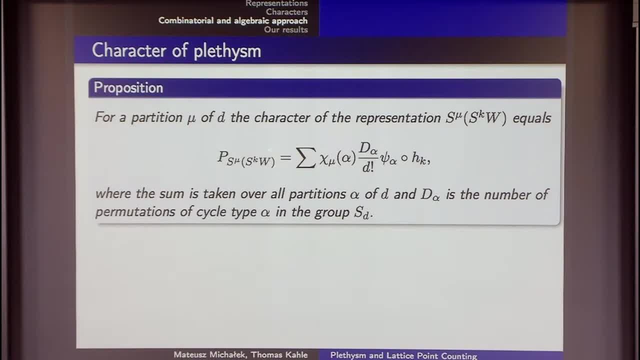 So this is the formula for the character of, of Pleiades, of ns, mu and sk. There are some strange numbers here, And let me. let me explain what are. what are these numbers, using the proof of this thing at the same time. 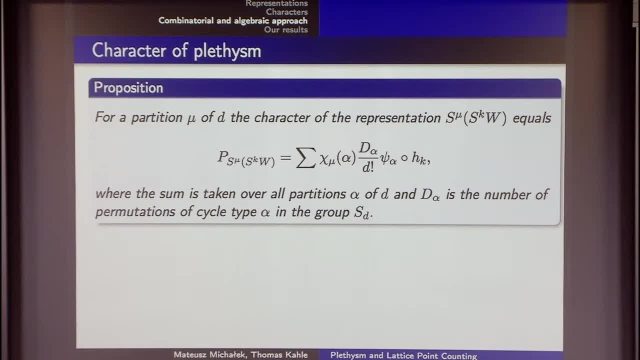 So a few numbers are expressed here. So the sum is over all alphas that divide d And d. alpha is the number of partitions of cycle type alpha. So if you have a partition of permutation- yes, sorry- of permutation, permutations of cycle type alpha. 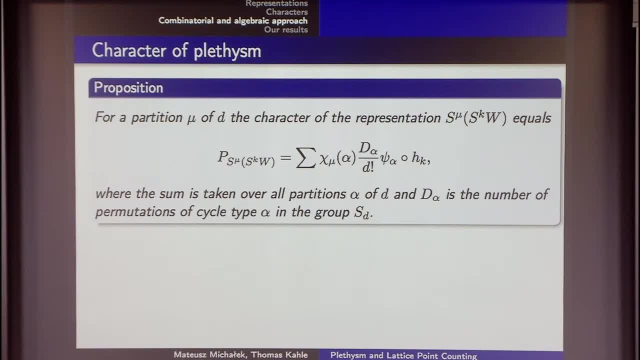 Yes, so if you have got any permutation, you can decompose it to cycles And you can ask how many permutations are with the same decomposition to to cycles. So this is d alpha And the proof is very easy. You can see that this is like a two-line proof. 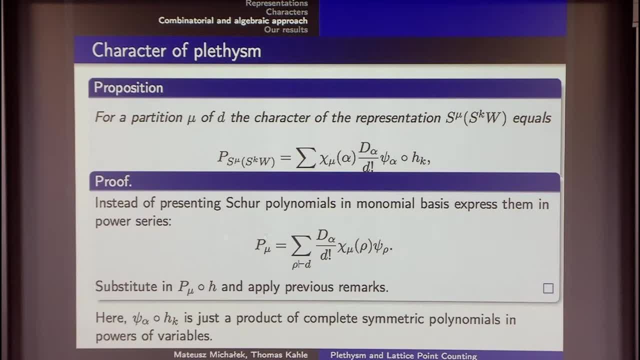 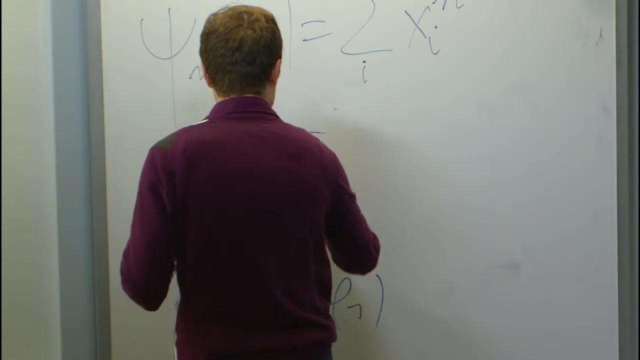 The. the thing is to decompose the character, the, the Schur polynomial in terms of power signs. So here rho is a partition, Rho is a partition, So rho equals rho 1 up to some rho s, And I define it just to be a product of rho i. 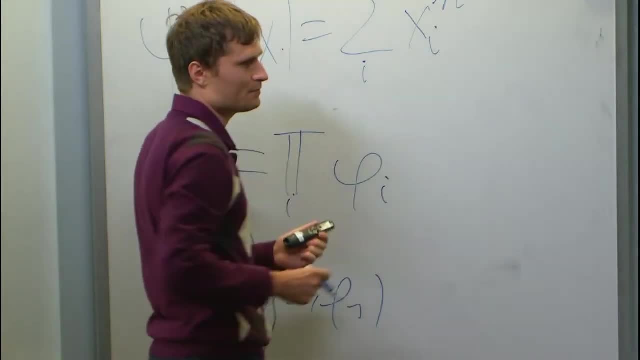 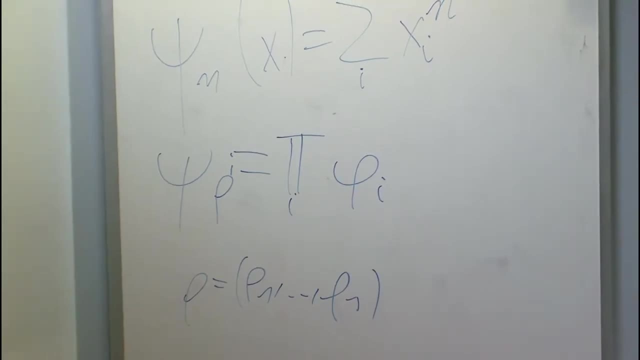 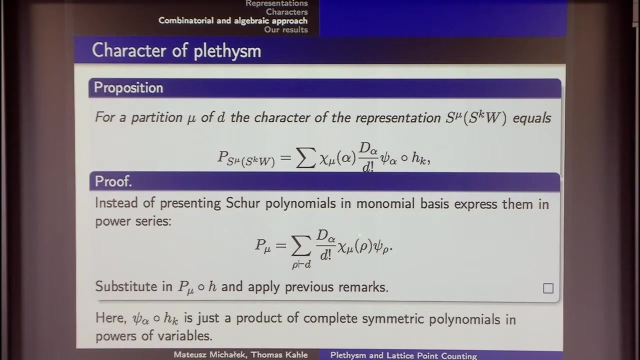 And rho with a number is defined above. So it's just a product of power sums. Is that some alpha in rho? Sorry, sorry, sorry, sorry In the sum. Up, up, up straight to the left There. 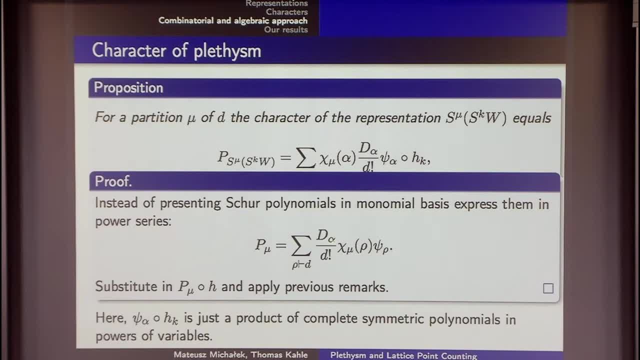 Yes, yes, yes, yes, yes, There there is no alpha here. I'm very sorry for that. And this phi is a psi. Psi of rho is defined as the product of the psi i. This is a polynomial defined there. 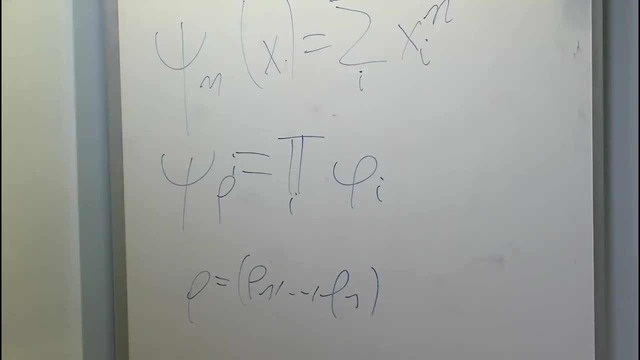 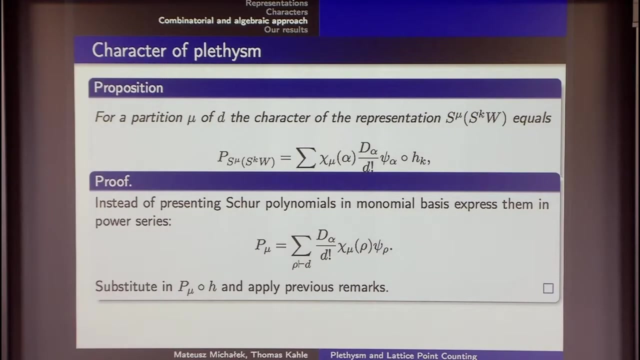 This is. this is just a number. This is just a number And I I'm I'm now going to explain this, Because I didn't say: what is this? Yes, I didn't say So. recall that partitions label, not only representations. 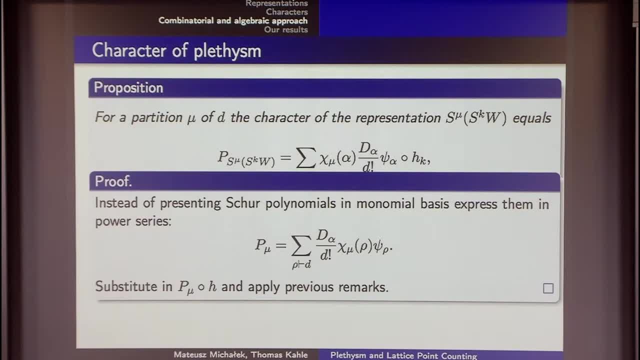 of the symmetric linear group. They also correspond to representations of the complete symmetric group, And complete symmetric group also have characters, And by psi mu I mean the character of the representation associated to mu, of an SD representation, And now I can evaluate it on a partition. 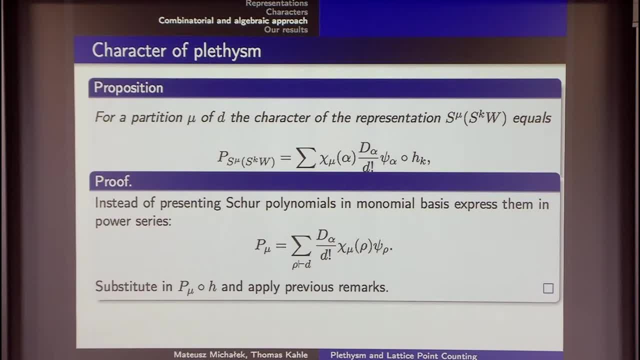 that represents a permutation, Because a partition represents a permutation up to conjugation, Because it defines the cycle type. Also, some people are nodding, but I think that not all people. Maybe there are some questions. So just to sum up, 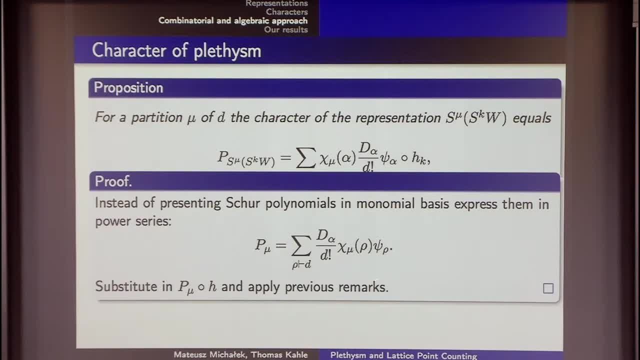 This is a formula to express the sure polynomials in terms of products, of power, sums with coefficients that are just numbers that we can understand and compute Dot. And now, using the fact that the platism is just an endomorphism of rings in the outer thing, 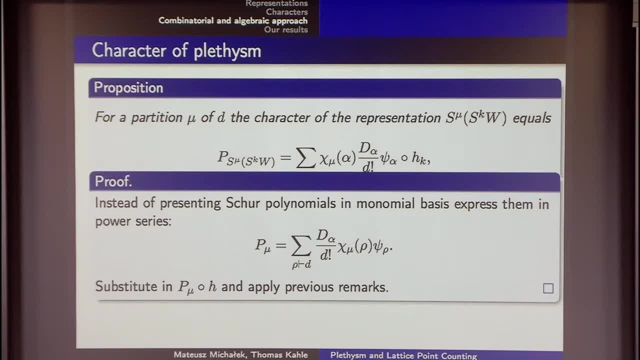 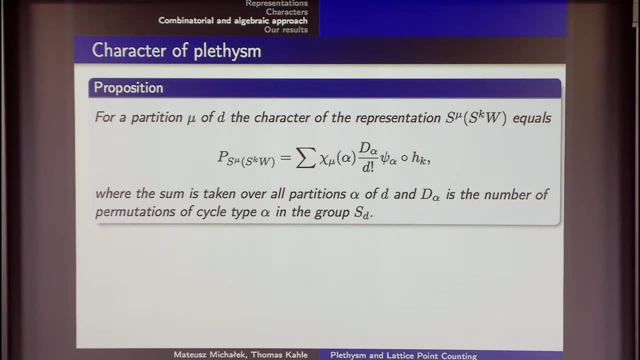 we can put it and compose it with the character of the symmetric power, which is just the complete symmetric polynomial, as we have seen, And we obtain this easy formula. What is d alpha now? d alpha is the number of permutations of a given cycle type. 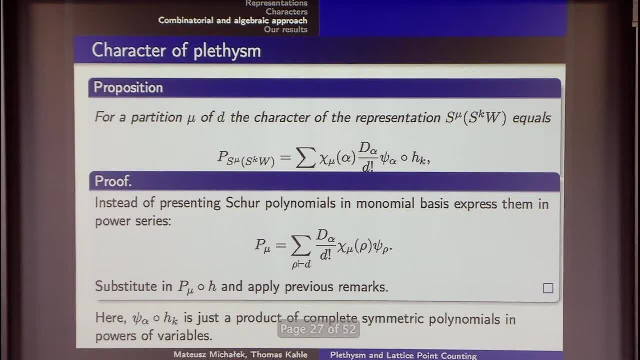 You can write a precise formula, but I think it's easier to just remember that it's a number of certain permutations. So basically, sure wide duality, right? Yes, You can derive it from. sure wide duality. Yes, you can do that. 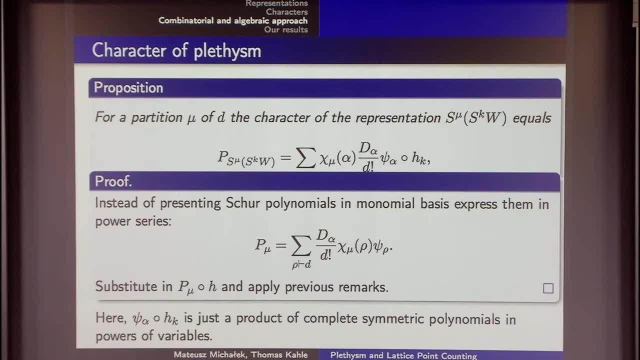 Although I always did it on polynomials Great. So at this point, when I think I learned it from Laurent, I thought the game is over for platism. We know the character, so we know the polynomial. What's the problem? 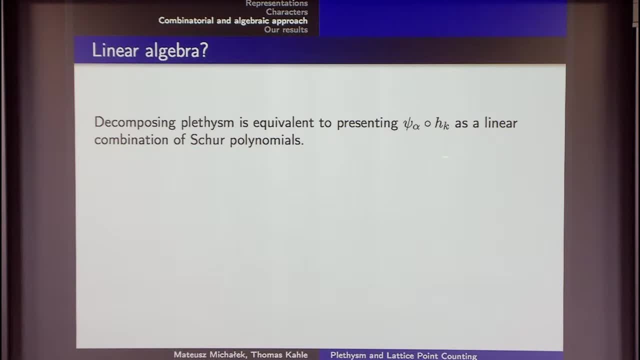 I mean we just reduced a very complicated problem. in linear algebra We have to understand this polynomial as a linear combination of sure polynomials And the problem is, I think, more or less the same as in Professor Popov's lecture: Linear algebra. when you are doing it, 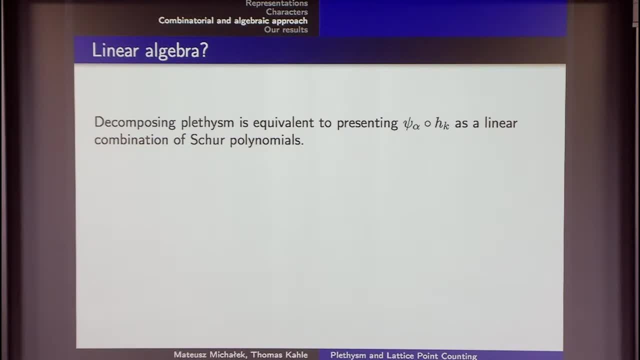 in coefficients of polynomials becomes hard Because there are so many of things. So this is the reason why this problem is not completely solved. I mean, you can try to do it, like combinatorically or using linear algebra, but the formulas become complicated. 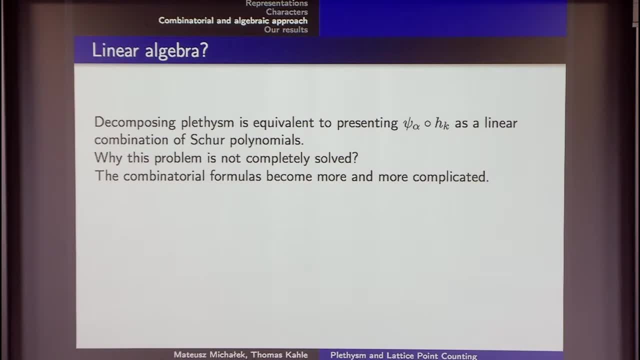 The computations become more and more complicated, But we still have our aim. We really want to understand low-degree polynomials in arbitrary polynomials. So we don't care if it becomes complicated, We have to do it. So what can we do? 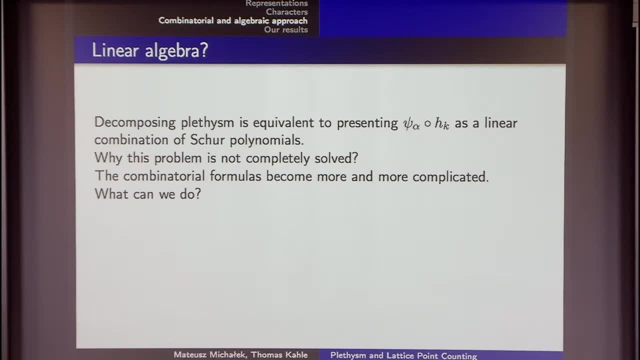 So I think there are two things in general that one can do in such a case: Either really aim to really obtain the aim using some new methods that people before us didn't use, or try to ask a different question, Maybe not an explicit answer. 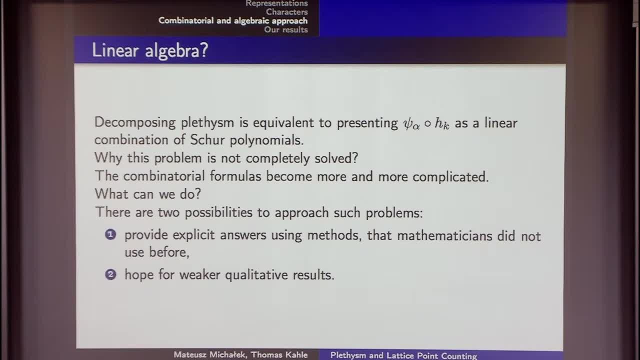 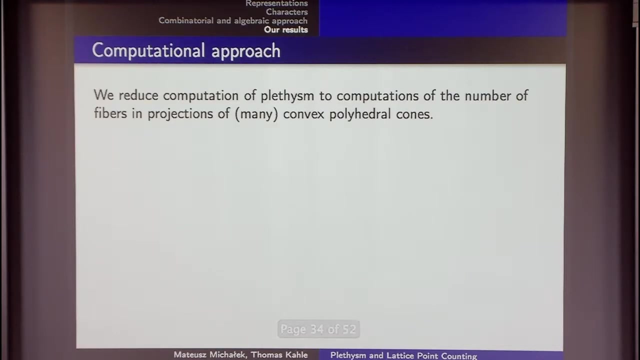 but something connected to the answer, And I will present both of these approaches, point one and point two. So point one: we have to use some new methods that people before us didn't have. So guess what will be the methods that people in the 80s didn't have? 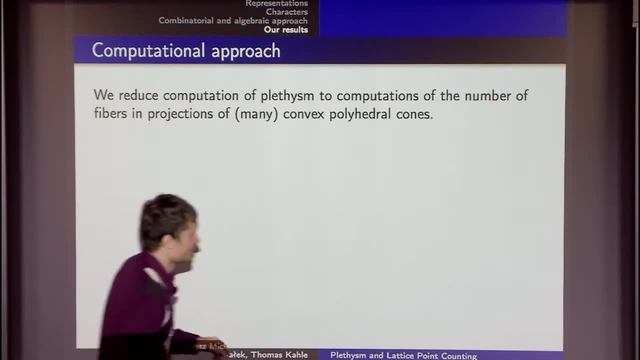 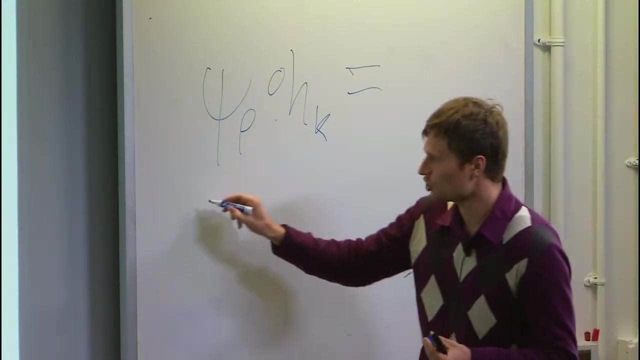 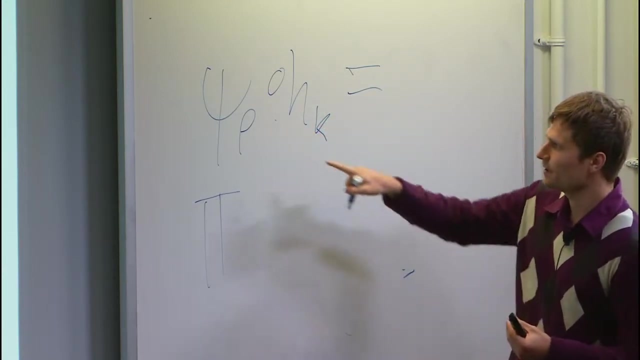 Well, the first problem is to understand is to understand this polynomial: Psi rho h, k. I don't know if you see what it is. This is just a product of complete symmetric polynomials. So, first of all, this is a product of psi rho i h k. 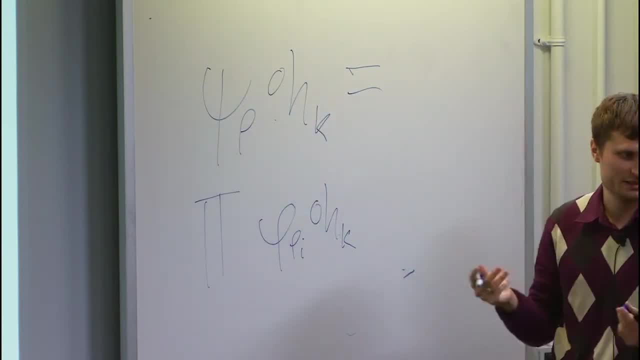 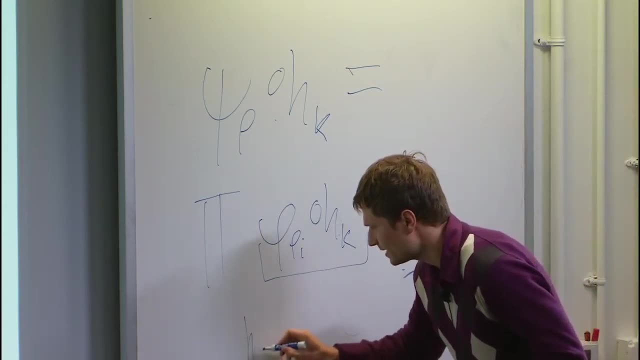 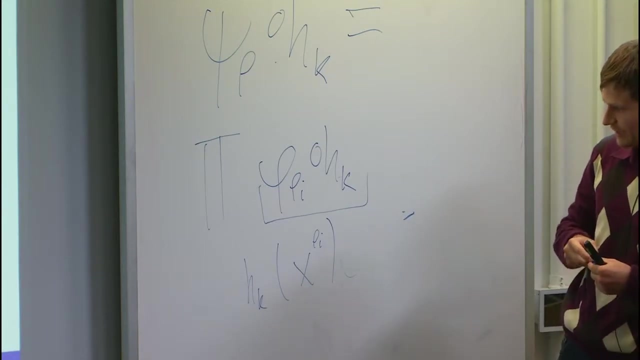 because I told you that the pletism is an endomorphism in the outer function. So we would like to understand this. but this is just h k of x to rho i, a complete symmetric polynomial of degree k in coefficients that are not variables. 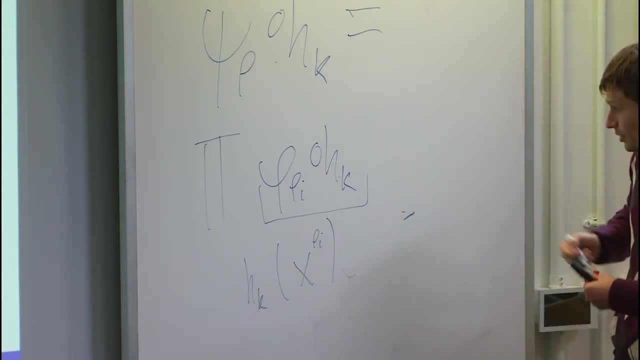 but powers of variables. So what are the coefficients of this coefficients? And we have a product of such things. How can we understand the coefficient? Well, let us translate it to a purely combinatorial problem, as a few speakers before me did. 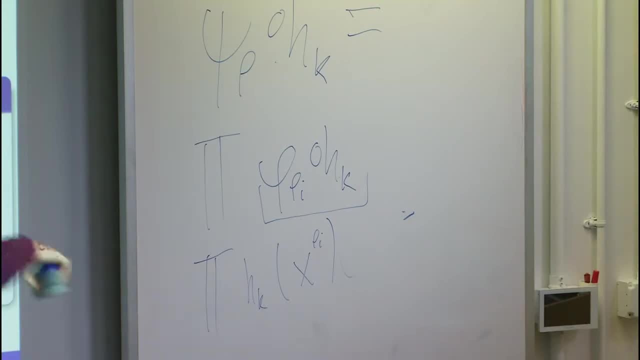 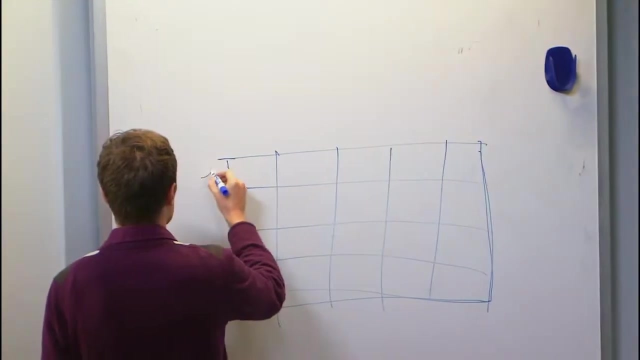 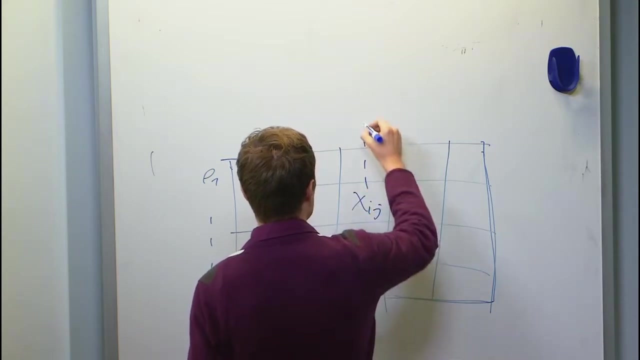 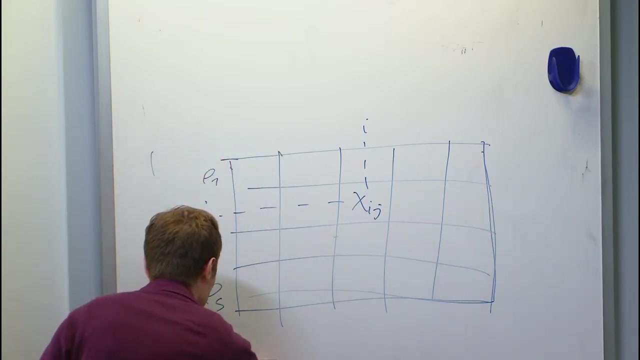 So you can immediately see that the coefficients of this polynomial are governed by the following combinatorial object: You take a matrix, Your matrix has got certain weights, And so the entries will be xij, And you want the rho sums to be equal to k. 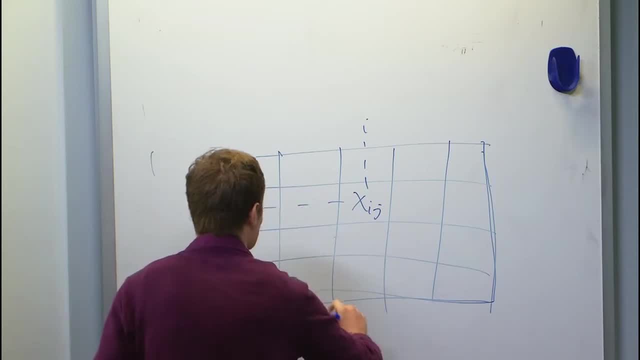 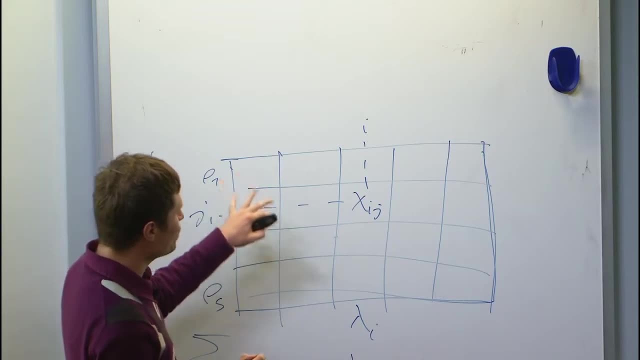 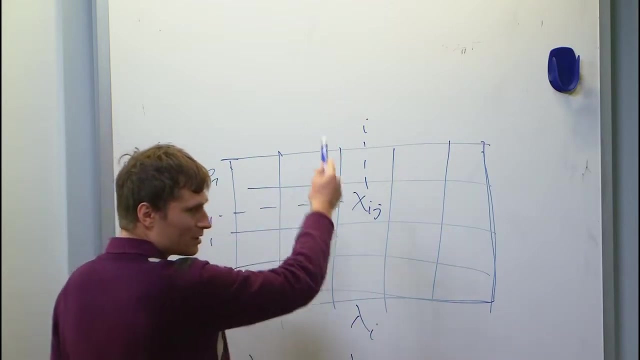 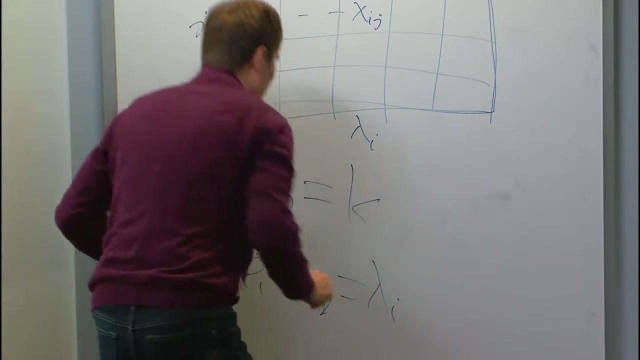 to a given fixed number And you want. So xij are numbers? Yes, numbers. We will be counting number of matrices with non-negative integral entries, with rows summing up to a given number and weighted column sums. weighted column sums equal to lambdas. 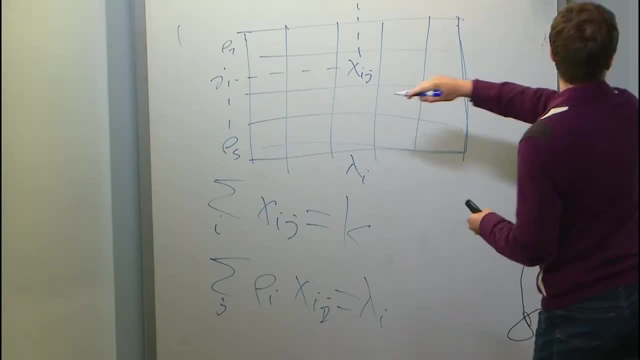 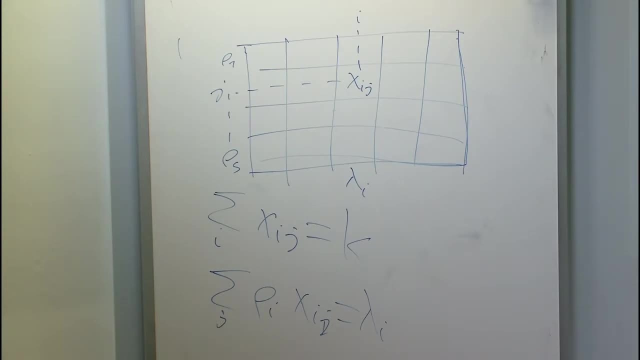 So you should write kj. No, the k is the same everywhere. It's hk. Oh, it's hk, Okay, okay. So This sort of tells me which monomials I choose in each of the products. Very, very easy translation. 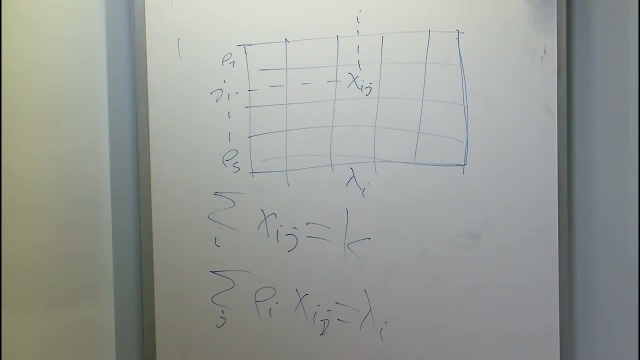 So this expresses: Oh, uh, The first one is the columns that are fixed rows that sum over j, And the next one is sum over i. Uh well, that depends how you number them. Here I gave i and here I gave j. 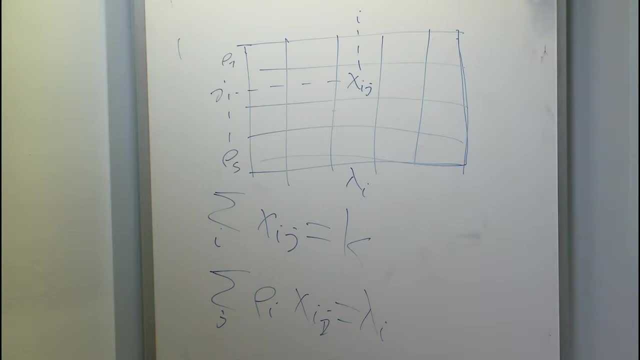 Sorry, Probably many mathematicians. So this is the arithmetic of the degree vector. Uh, yes, Yes, yes, yes, yes, yes. I just encode the coefficients. Very simple, But the good thing is that now we can apply new methods. 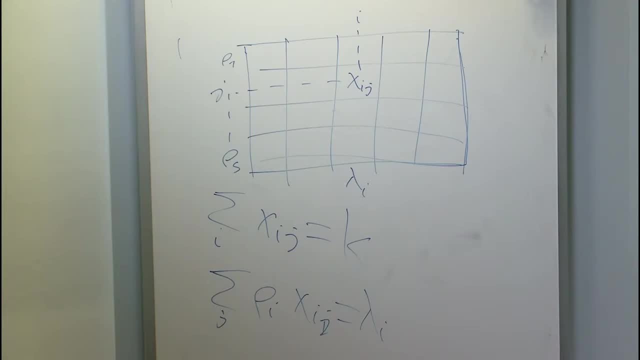 that people didn't have in the 80s. I mean, this is a perfect job for a computer Because this is a polytop. This is a polytop and there are new algorithms. People developed new algorithms to compute such things In particular. 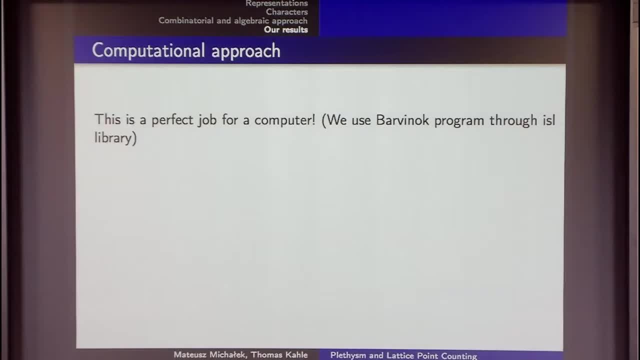 there's a Barvinok program which greatly solves the problem of computing parametrically, of computing parametrically the number of points in a cone. So I had a few questions about the Barvinok program because it was mentioned during a few talks. 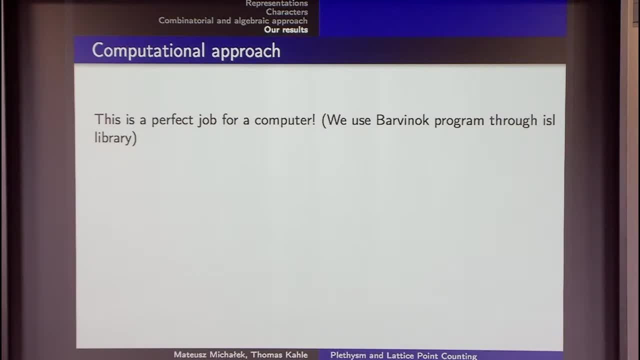 We use it for ISL library. It's still under construction, but it works already very, very well. So what does Barvinok? We have a polyhedral cone, We have a poly. So this is a three-dimensional polyhedral cone. 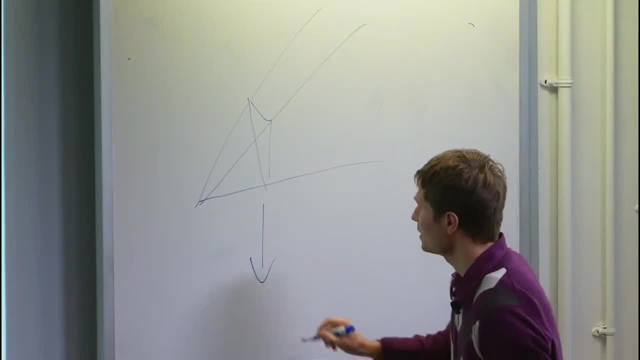 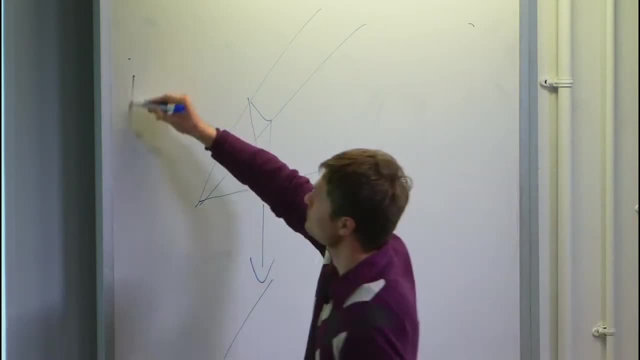 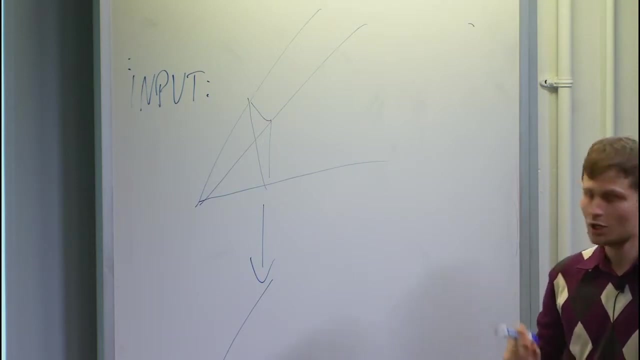 And this is, And we have a projection, So I will be projecting it to a two-dimensional space, And this is the input, And the output is a counting function of fibers. So I would like to know what is the cardinality of a fiber above a given point? 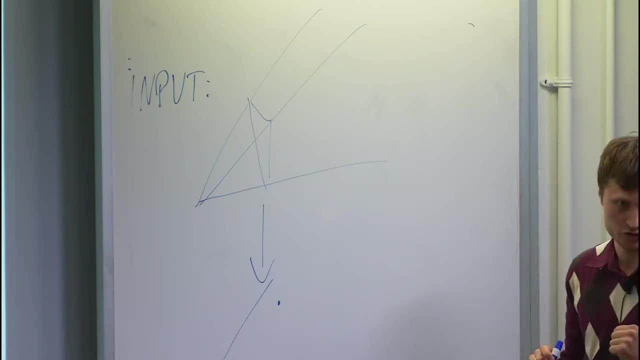 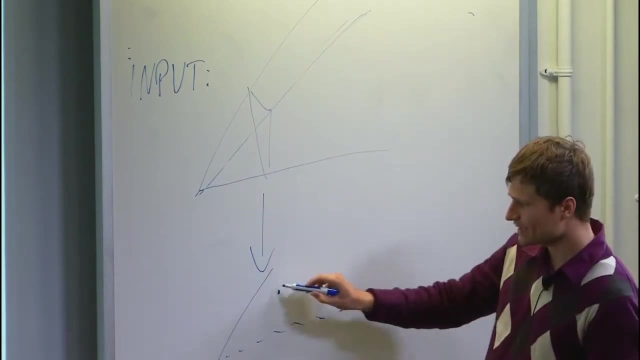 But I don't want a number, I want it as a function. So what do I get? Notice that this ray projects here And of course, I get a different function on this piece and a different function on this piece because the facets 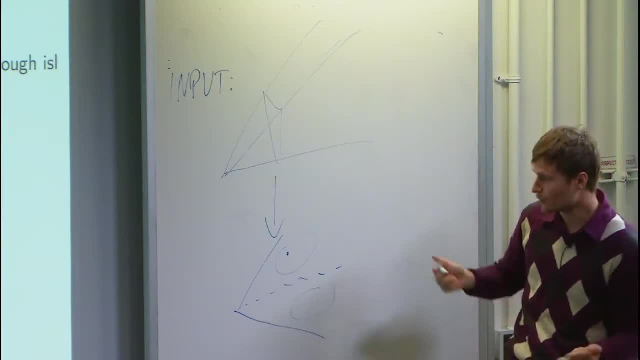 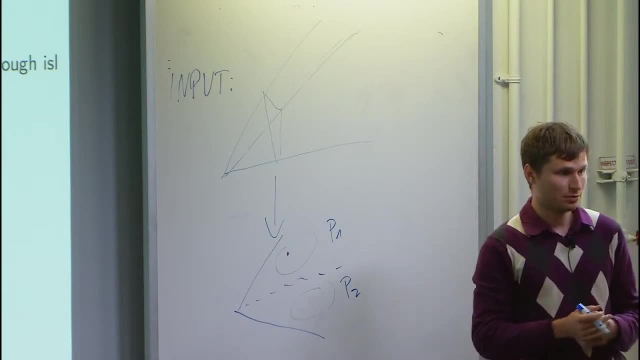 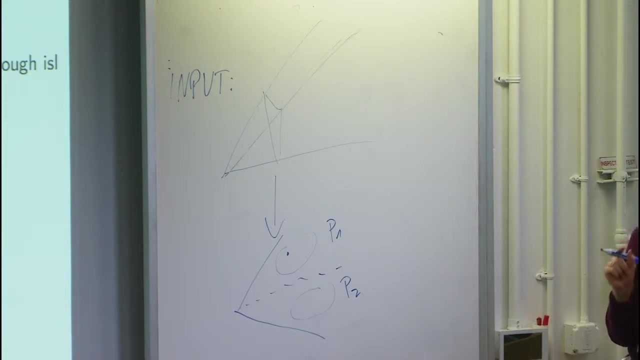 supporting the cones are different. Yes, So I get a quasi-polynomial here and a quasi-polynomial here. What do I mean by a quasi-polynomial? I mean just a polynomial, but the coefficients depend on parameters, modulo a fixed number And this is the output. 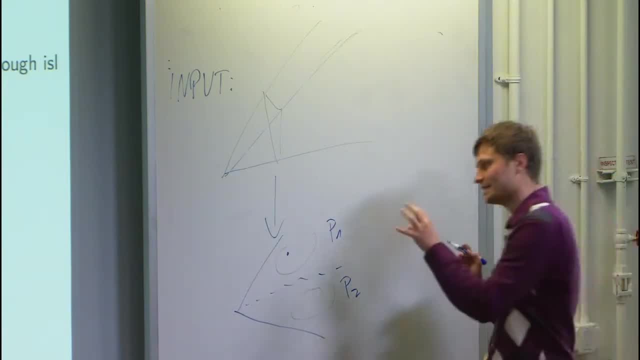 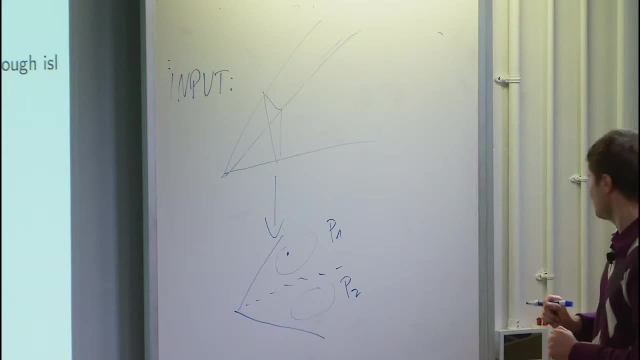 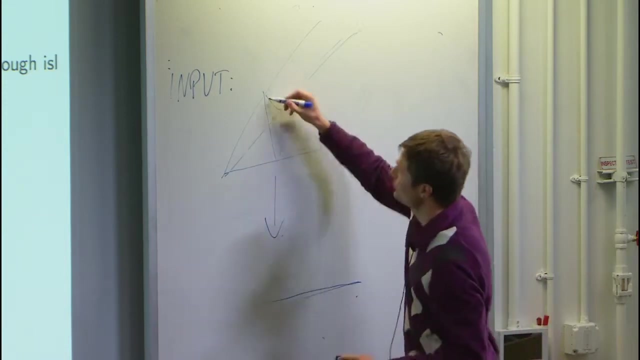 of a Barvinok. He gives you the chamber decomposition and he gives you the quasi-polynomial in each chamber, Just to check if the audience is with me. what would I get if I would project it to a line? So this polytope? 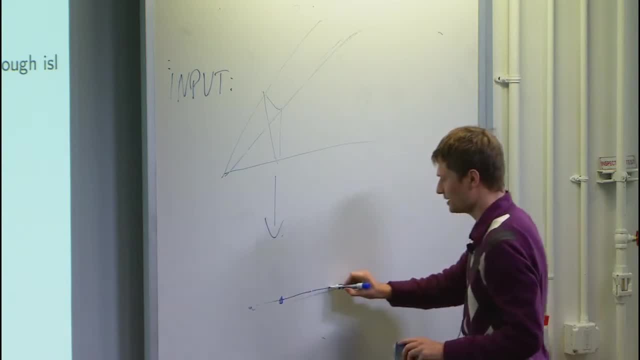 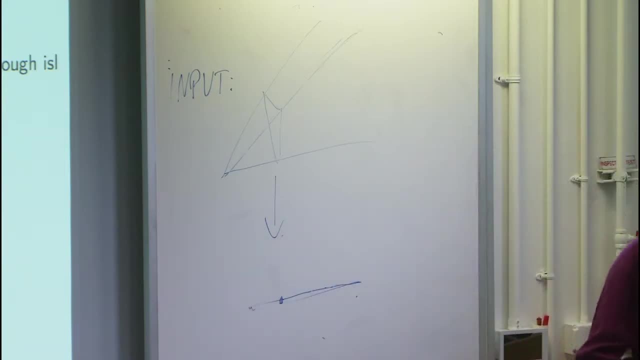 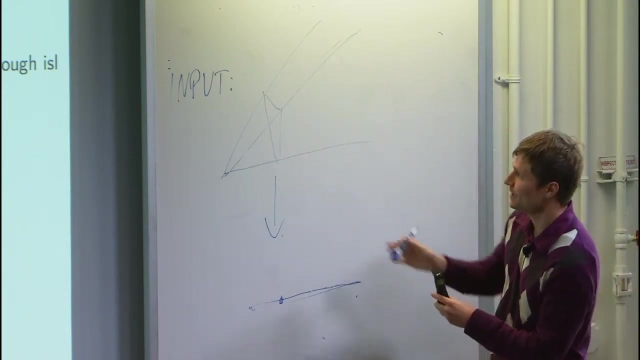 projects to a point and I'm counting the cardinality of a fiber. Yes, Someone is with me, Great, OK, So I project it to the line and I assume that there is a polytope at height one and then there is a dilation of this polytope. 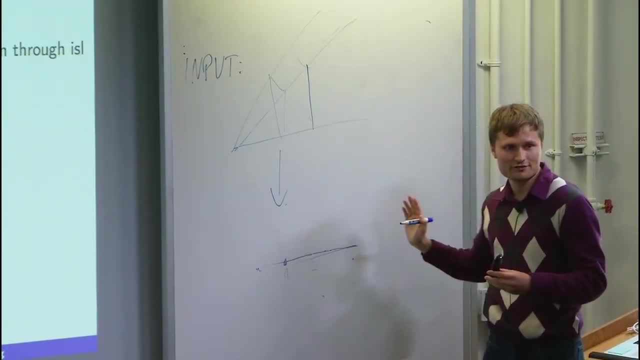 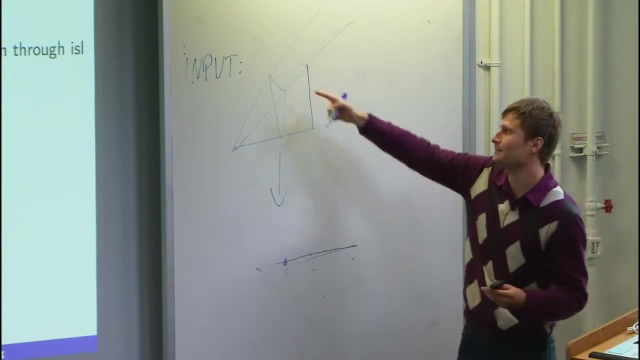 at height two. So in fact, the projection function counts the number of integral points inside the dilations of the polytope, And this is I mean depending if this is rational or integral. this is either a polytope or a quasi-polytope. 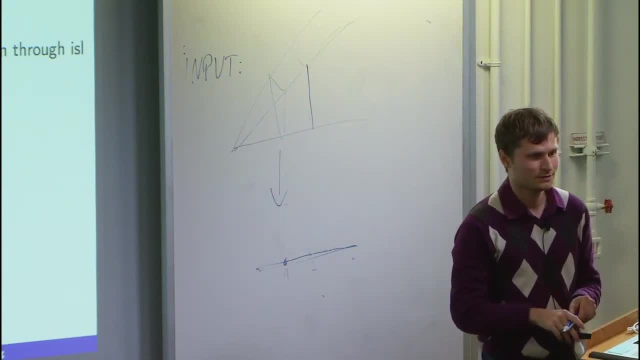 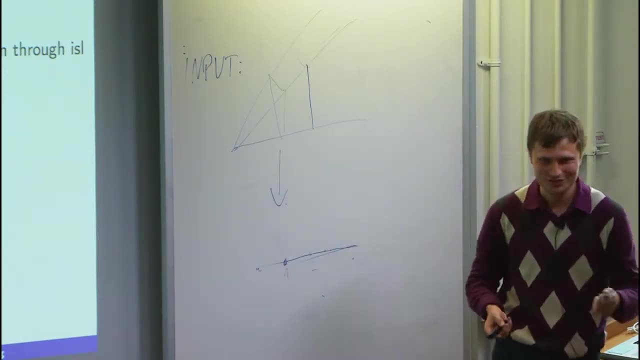 The Erhard-Hilbert. Well, it's a polynomial. but whether it's a polynomial- Yes, whether it's a polynomial or a quasi-polynomial depends if this is integral or rational. Great, So we obtain. We obtain a lot of cones. 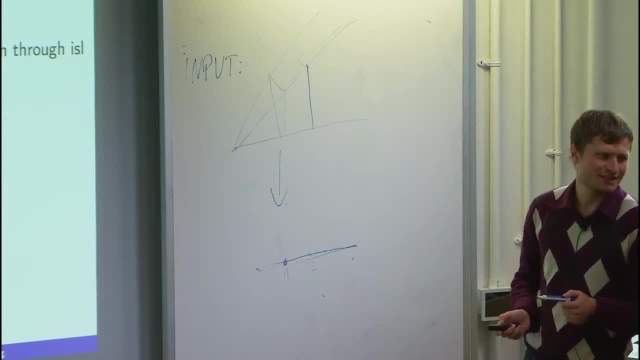 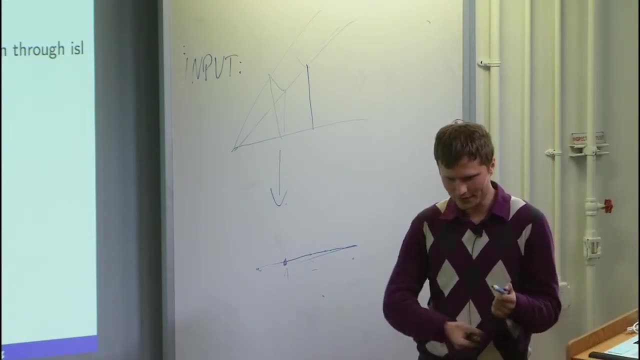 We have to project them. So I cheated here a little bit, because I told you how to understand the coefficients of the, of the, of the character of the plethysm, but coefficients are not enough to to to understand it as a decomposition. 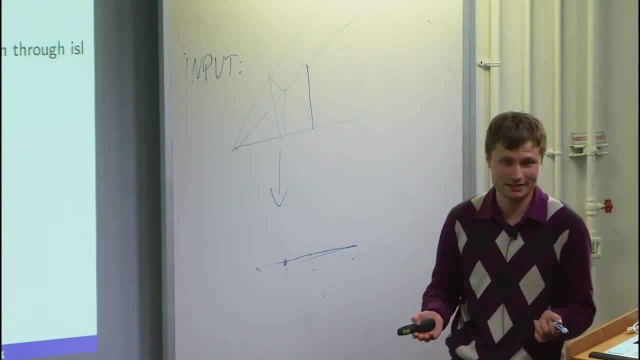 of sure factors. but there is a standard trick that was mentioned during the previous talk and many other talks: You can, You can. You can call it in many different ways a finite difference operator. It amounts to multiplying the number and it amounts to multiplying. 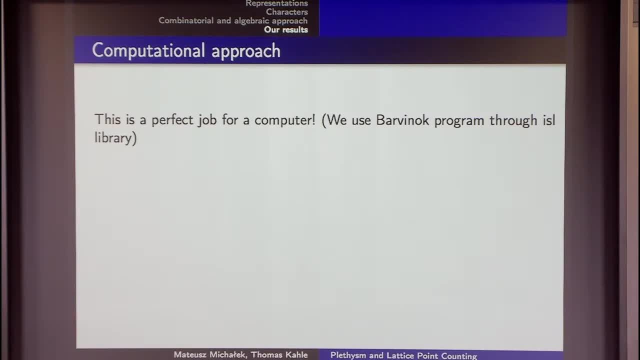 your polynomial by the discriminant and then looking for the particular coefficient. there Also a job that a computer does very, very well for you. And we get explicit answers where mu is any partition of four or five. So in particular, we also obtain an explicit answer. 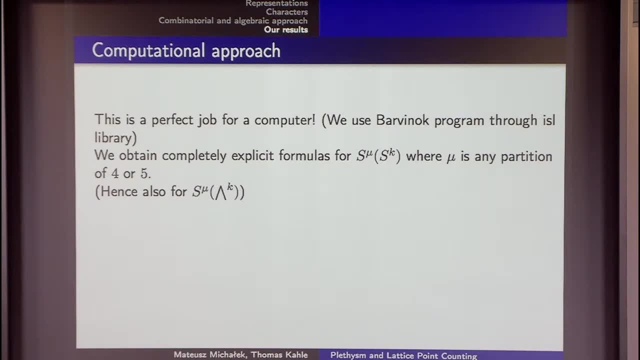 for s mu of wedge k. Of course, don't try to implement it as I did it in the previous talk, because the computer will break. but after a few tricks you can. you can do it with, with, with with, without problems. 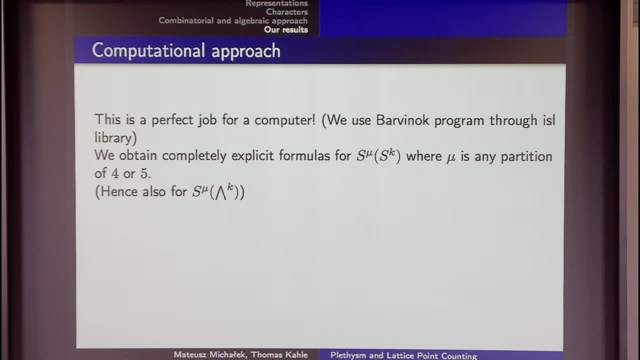 No for any k, A formula for any k. So I I should mention there are 1,000 programs and the best one is Li to compute for fixed mu and fixed inner thing. But we don't want that. We treat k. 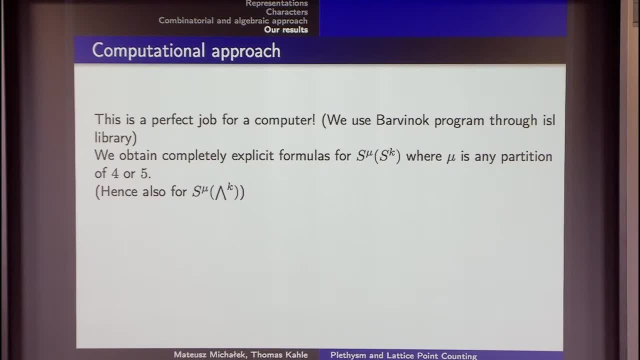 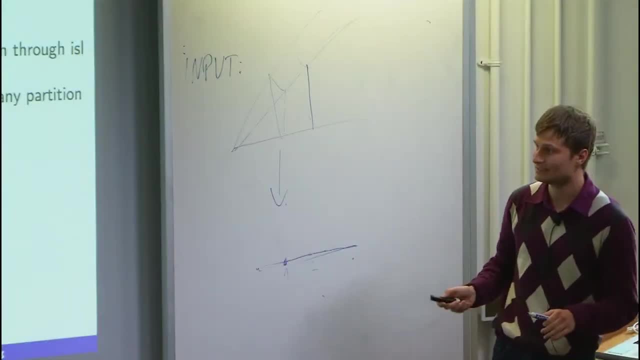 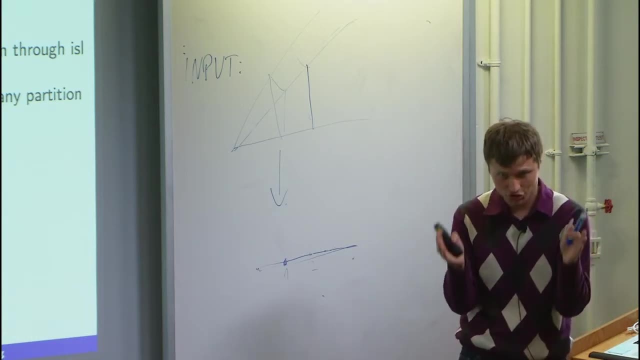 as a parameter, in it's a parameter And our formulas are completely explicit. So it gives, we obtain a decomposition of the space of k's and lambdas, the domain, and finite decomposition into chambers, and in each chamber you get a quasi-polynomial. 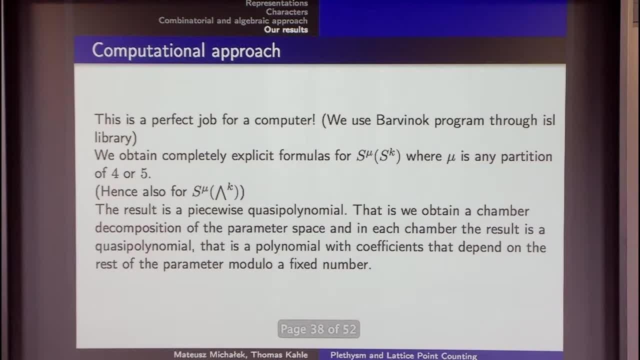 explicitly given by the computer. Yeah, so this is what. this is what I just said. Yes, so we have. we have a space in the domain. is k lambda? you don't need both, but let's say we have both, and then you have. 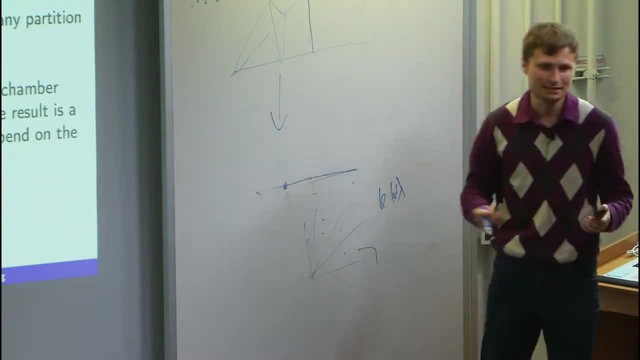 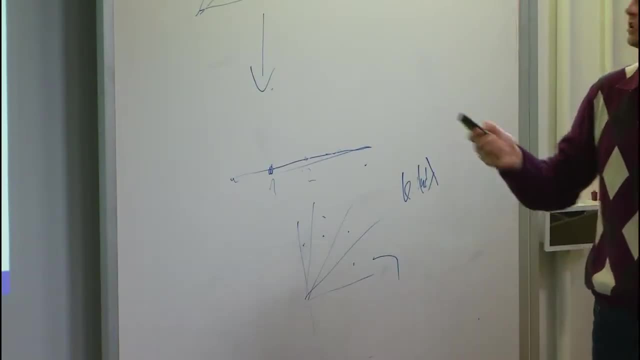 a chamber decomposition and in each chamber you get a explicit quasi-polynomial that gives you the answer to your problem. So if you would like to then know, yeah, I will, I will pass later what you, what you can explicitly do with. 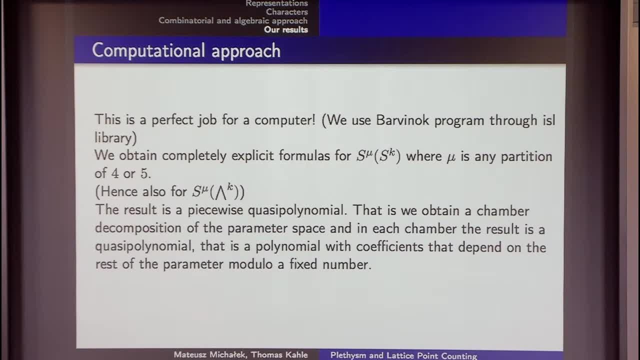 with that. Sorry, The number of chambers would be huge. Oh yeah, Really that huge. We've got numerics. It's like: Well, as mu grows, of course, As mu, you have the most 4 and 5.. 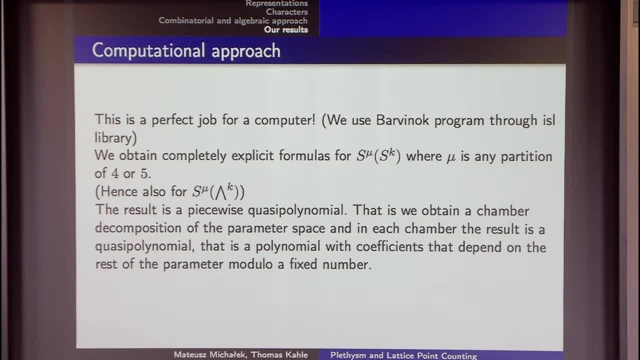 I know. So that's what, Yes, Yes, That's what keeps it still reasonable, I guess like 120.. I don't remember That's a, Sorry, That's a, I don't know. 100? Yeah. 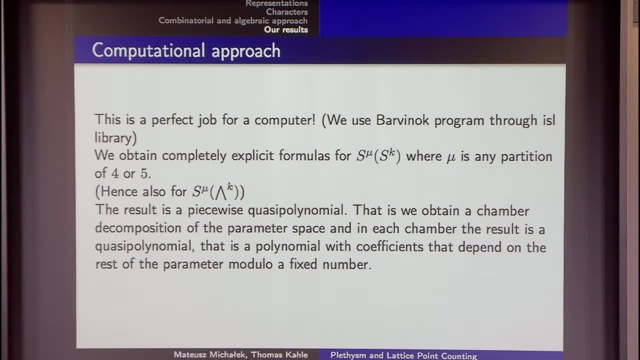 Not, Not, I mean it's, it's. That was actually 75 or 75 already. Yes, because they are writing it explicitly, not as a formula, But we've got s5 of sk for any k, Any k. 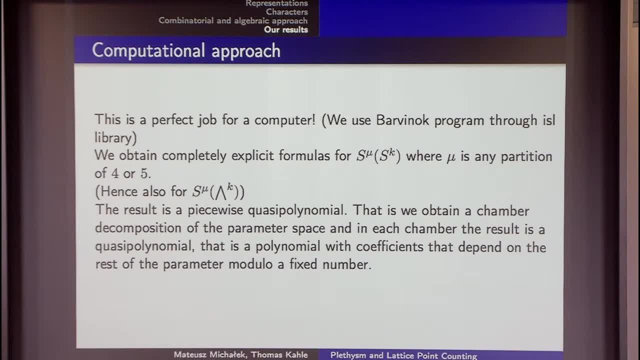 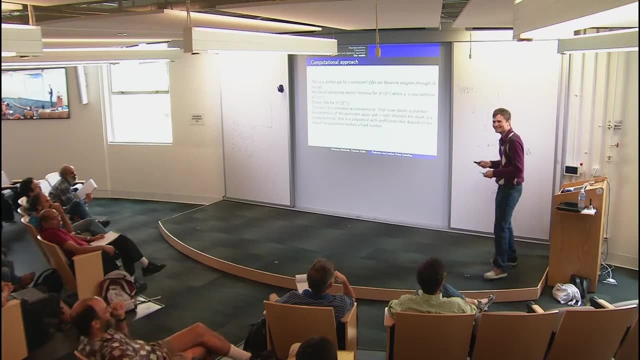 As a function in k, For example, for me, partition of 4, how many chambers do you get? I have to check in my. We have. I mean 100.. I get something between You use projection once or many times. 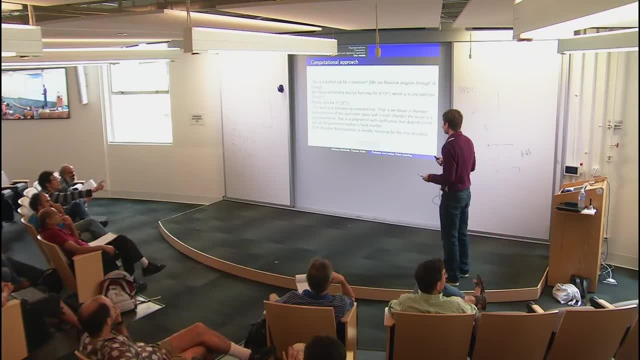 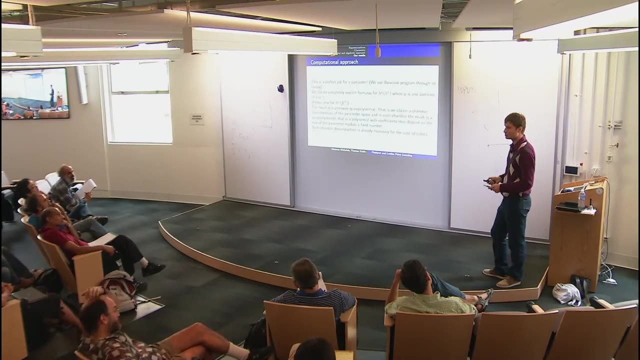 Sorry, Oh many times. Number of mu boxes: factorial. And I didn't show you any chamber decomposition, because for quadrics there was no chamber decomposition, But already for cubics you need this chamber decomposition. So there is a different. 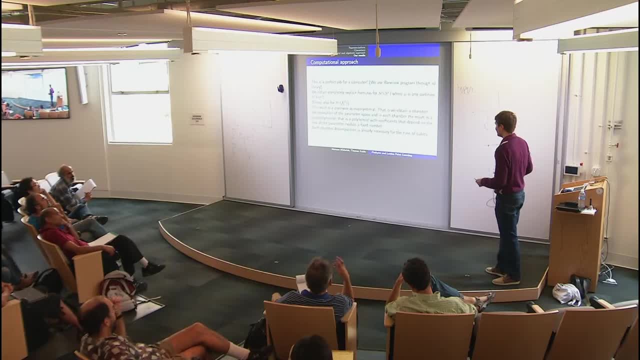 formula depending on inequalities. So of course there is a different formula. This is a quasi-polynomial, depending on the rest, modular fixed number. So if one doesn't care how you got the formula, there is a precise formula for decomposition up to s5.. 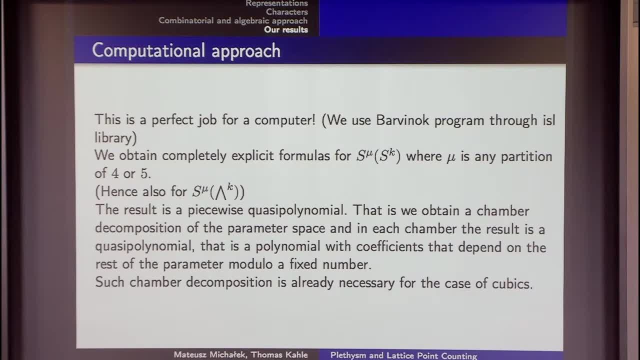 Yes, Is that what you're saying? Yes, Yes, Even smu, where mu is any partition of 5. s5 of sk. there is a formula in k. So not even for fixed k, Parametric in k. So 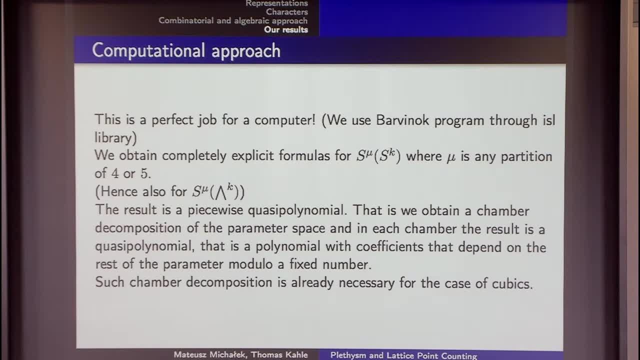 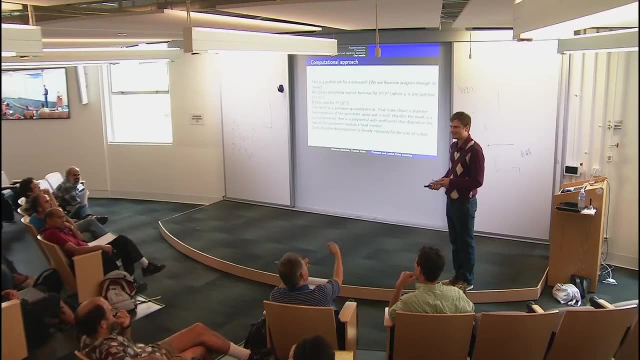 we understand quintics of any polynomials. No, Yes, So this is this trick that was mentioned by it was called sure something. I mean you multiply by the discriminant multiplicities. We are not cheating. Yes, That I didn't talk. 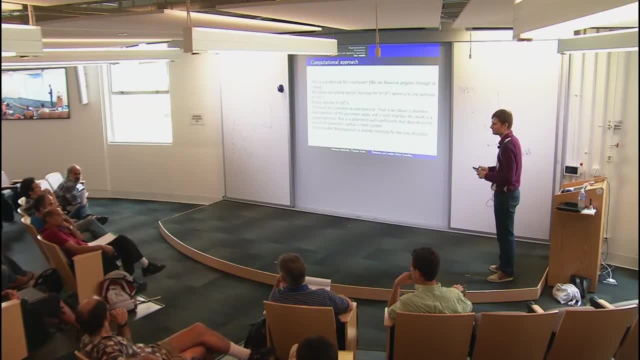 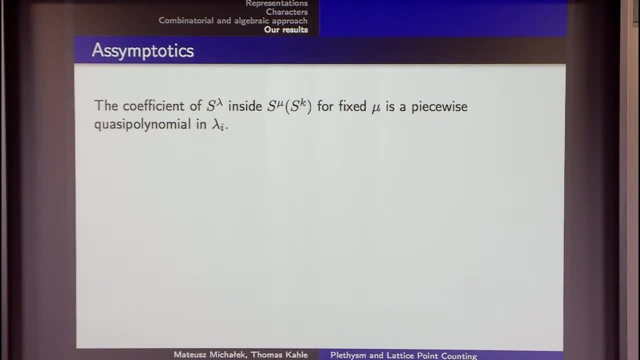 about: Yes, We did that. Yes, Okay, So so, so, but this is only half of what we did. I told you that there is a second point. You can try to understand things not explicitly, but, for example, 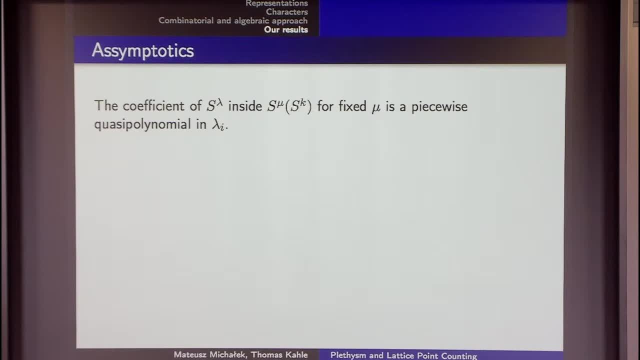 the asymptotics. So I already told you that this thing is a piecewise quasi-polynomial for fixed mu in k and lambdas. So for me there is a very natural question: What's the leading term of this quasi-polynomial? 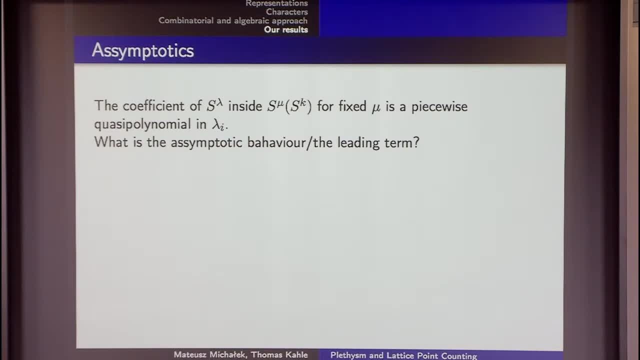 Can we understand it? And when you are doing combinatorics, you immediately see that there is the candidate for the leading term And- and you are sure that this is your leading term. And then you start looking at the literature and you find that 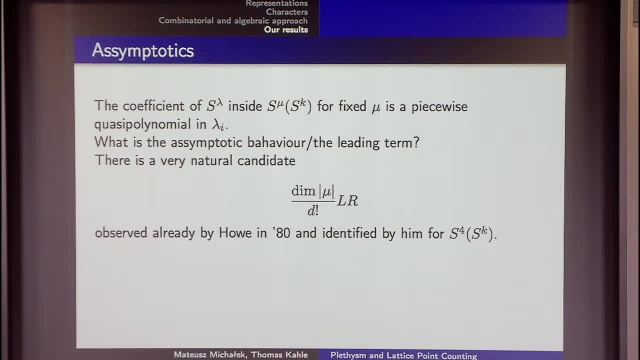 people before you also identified this leading term and they also were sure that this is the leading term, but it seems no one really proved it. I contacted like 15 experts, I guess, and R is Littlewood-Richardson. 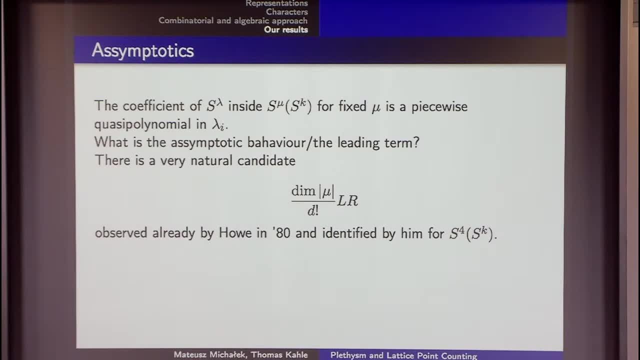 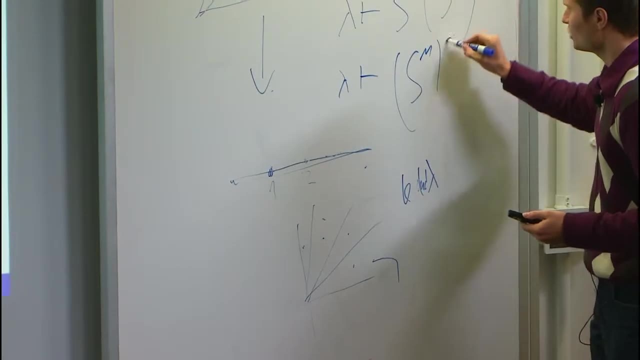 That's a big name. It's really coming from Pieri's rule here. Yeah, So more or less, if you want to understand lambda in S mu S n, you should understand lambda inside S n tensor, the weight of mu. This is much. 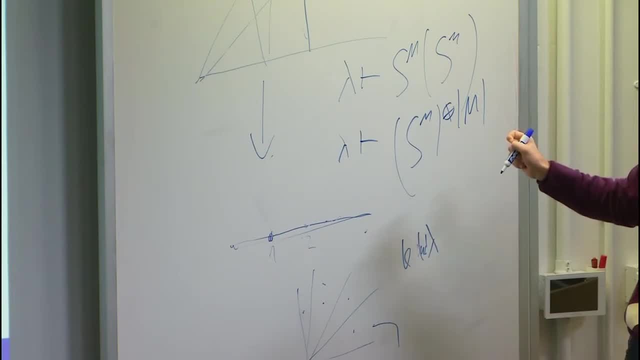 easier because this is just a number. It's the number of fillings of a tableau with Yes, yes, yes. but in this case it's like even easier because it comes from Pieri's, because it's a symmetric power. 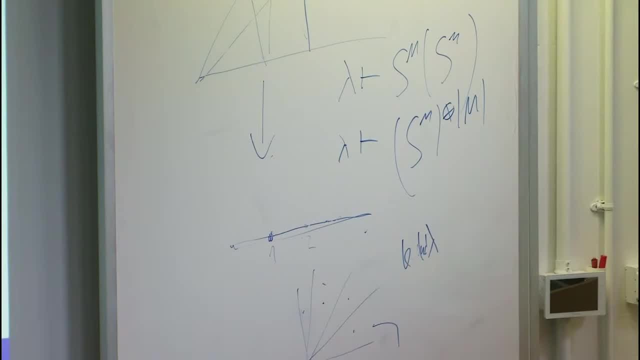 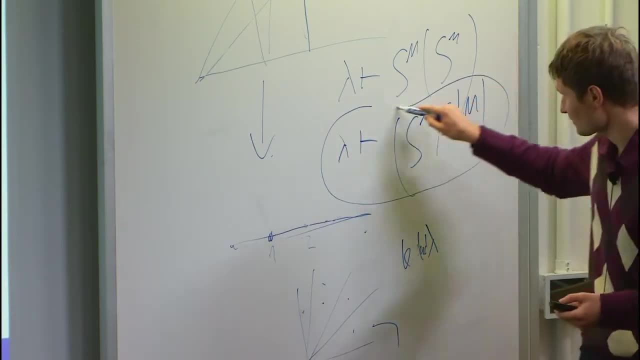 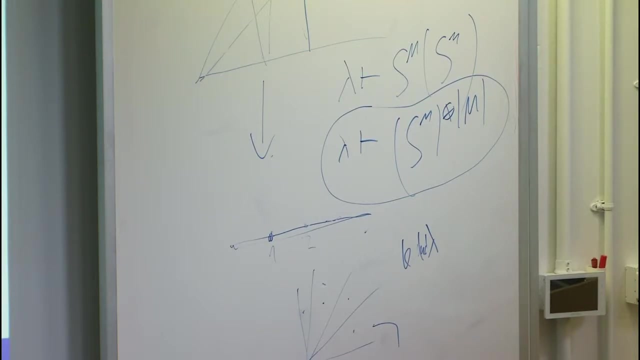 Yes, yes, yes, I call it the Pieri's rule. yes, but it is yes, yes, yes, yes. this number, but it's not a leading term. It's connected to the volume of the polytope. 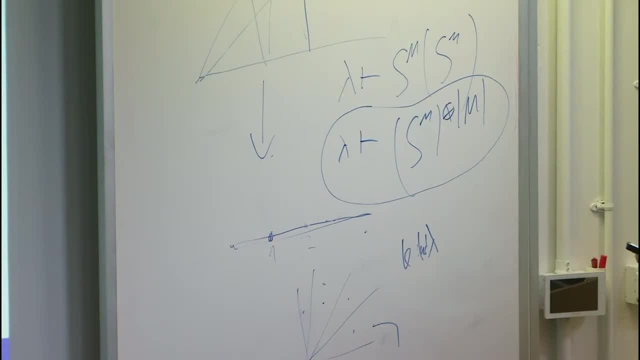 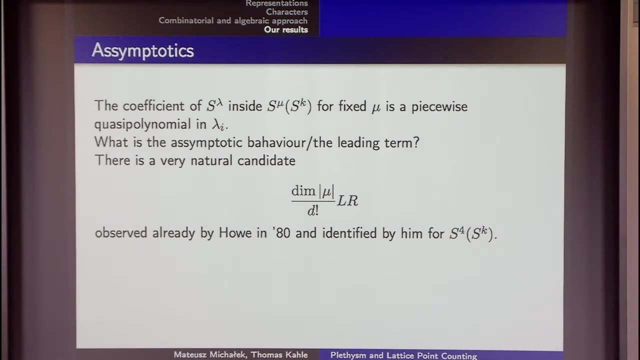 And then, if you want to understand the multiplicity here, just multiply by this number: Dimension of mu is the dimension of mu as a representation of the symmetric group. Okay, This should be. I guess many experts probably probably should feel. 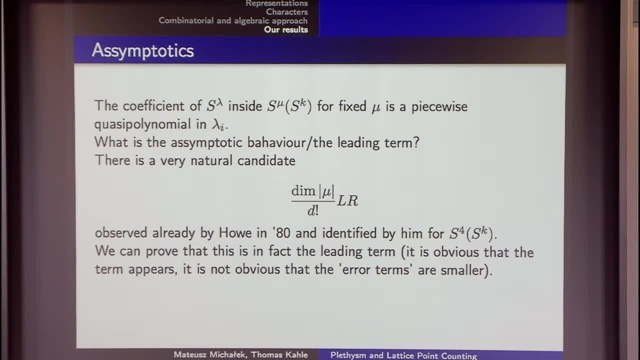 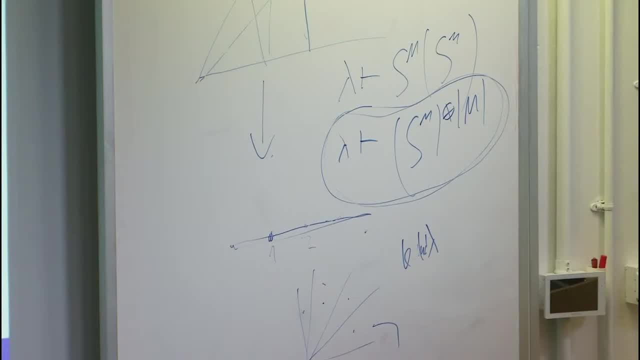 that this is obvious. I LR is, is, is from Littlewood Richardson, by which I mean, I mean I mean the term, the term in the tensor product. So what's the multiplicity in the tensor product? 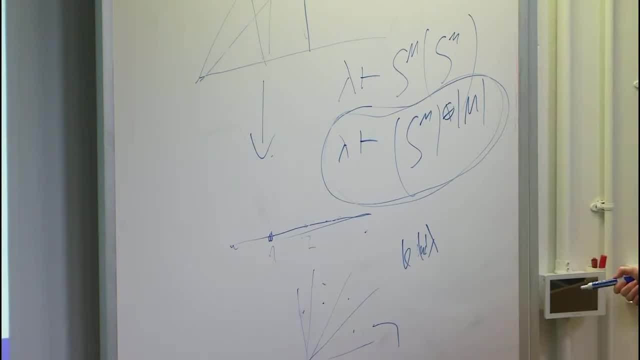 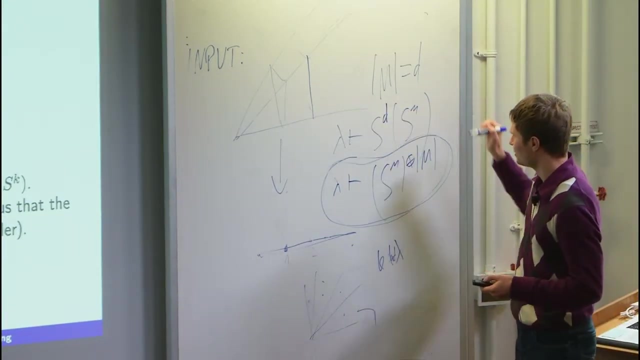 Of what? Which lambda, LR of lambda in there. Yeah, Yeah, Correct, Yeah, So so it's what was d, now d is is is mu. Oh, oh, size of mu. Yes, So, for example, for symmetric power, I mean, imagine that this is just the symmetric power, so that this is just D. 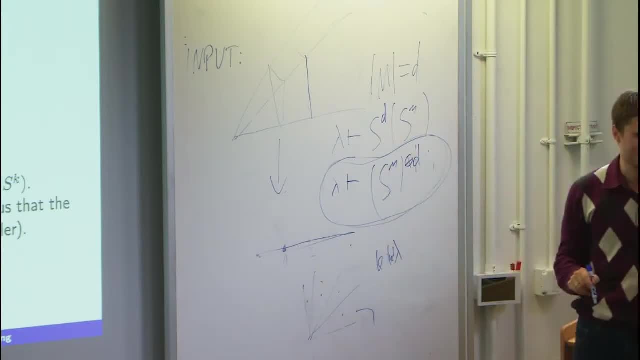 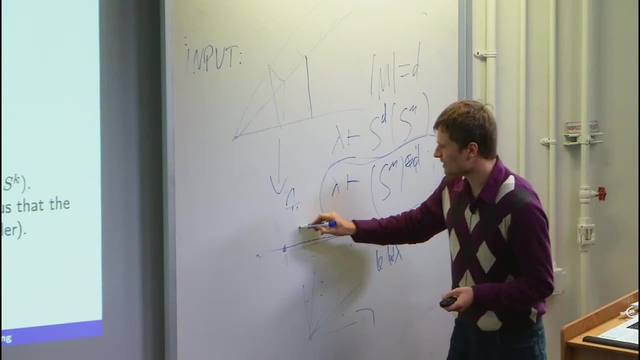 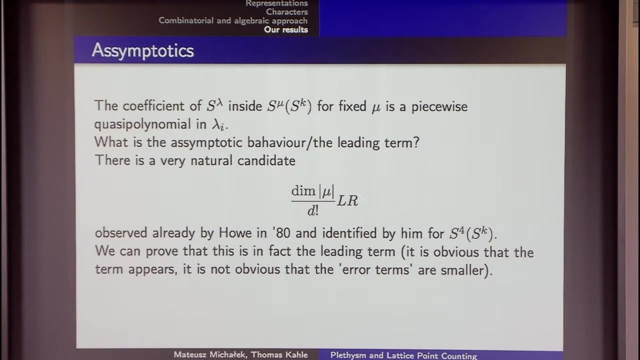 Well, what's the difference between a tensor product and the symmetric power? If you take an arbitrary tensor, if you symmetrize it more or less one over D factorial things will fall here. And if your partition is just one row, then this is just the trivial representation that has dimension one. 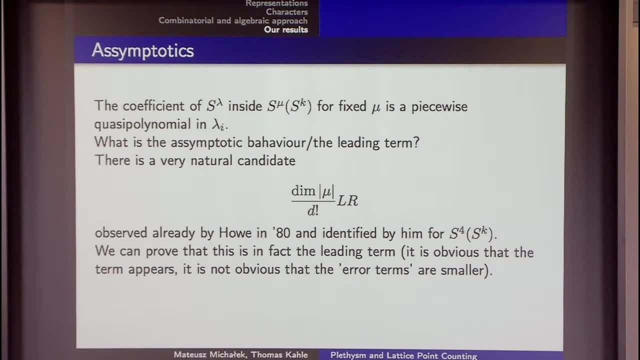 So you see that this is very intuitive. So we also prove it And I will be very happy to discuss with experts because maybe I still believe that there should be a very easy, not combinatorial, but a representation, theoretic proof of that. 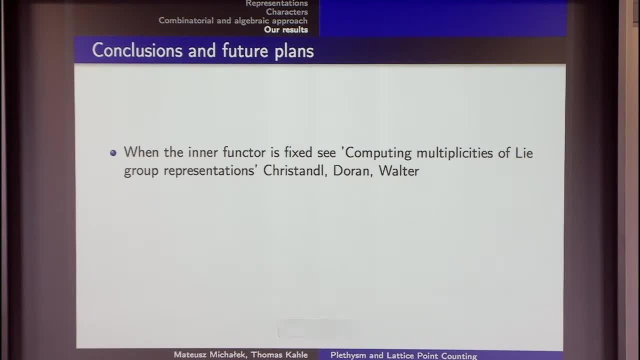 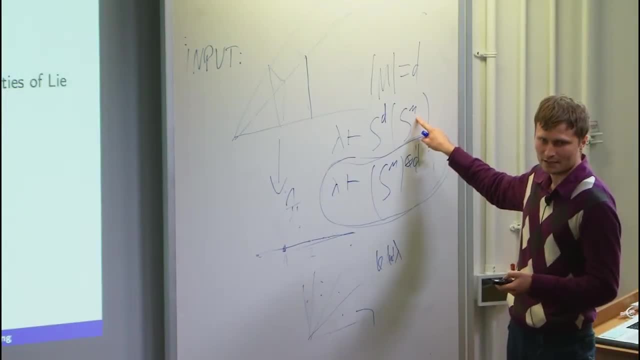 So conclusions and future plans. There was a talk by Matthias. So what's the difference with the talk by Matthias? He was changing the degree, keeping the inner functor fixed, So he had like one variety and changed the degree of polynomials. 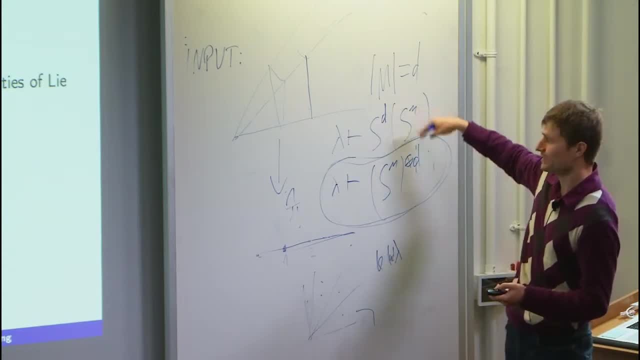 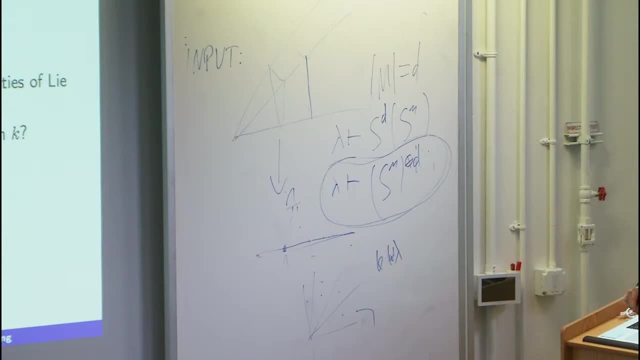 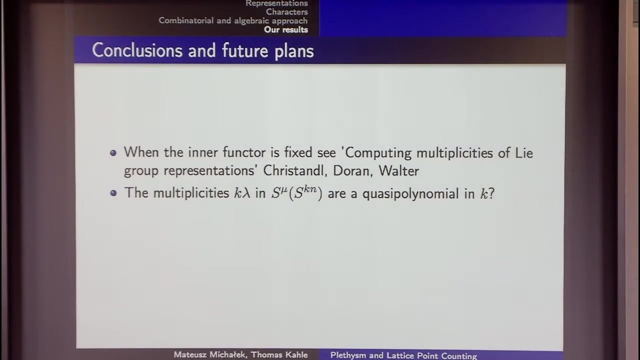 I'm doing the other thing round. So I'm changing the variety, I'm changing the polynomials, but I'm keeping the degree. So, after talking to Laurent and other people, it seems that this question mark should be a dot. 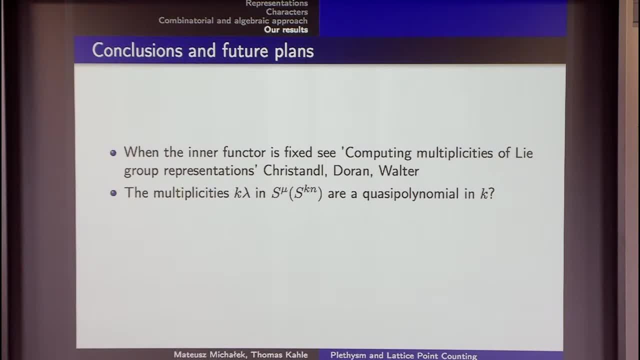 So from combinatorial formulas it's very clear that this should be a quasi-polynomial for large K. But it seems, It seems that it's a quasi-polynomial just from the start. So it means that you can understand the plethysm just by understanding it: asymptotically for very large values of K. 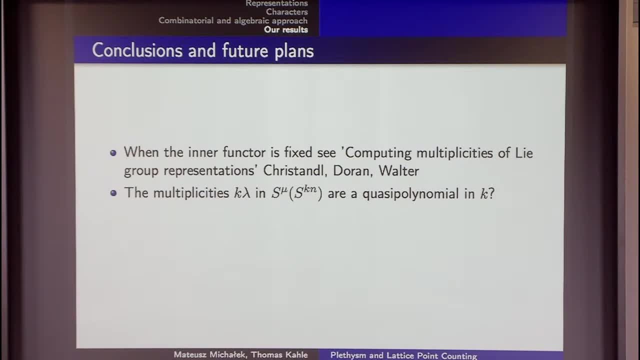 Because a quasi-polynomial is determined by finitely many values. So if you are able to understand it for large K, you can deduce the quasi-polynomial and understand it for small k. So I hope this will be a work in progress with Laurent. 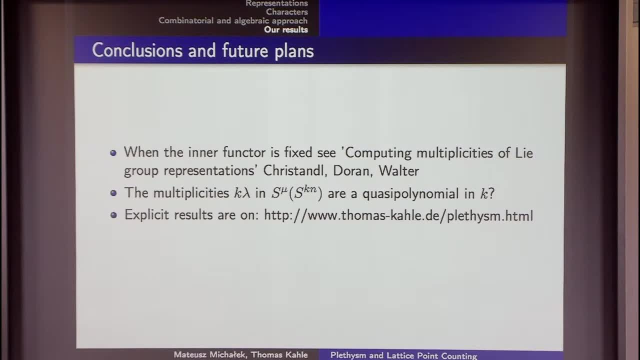 Oh no. no, there's a question mark, I see. I see. Well, Laurent and Matthias made it a theorem already, I think. So if you are interested in the explicit decompositions of S5 or S4 of Sn, this is the webpage we set out for it. 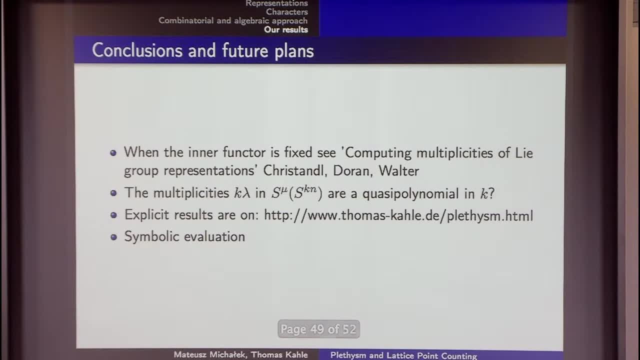 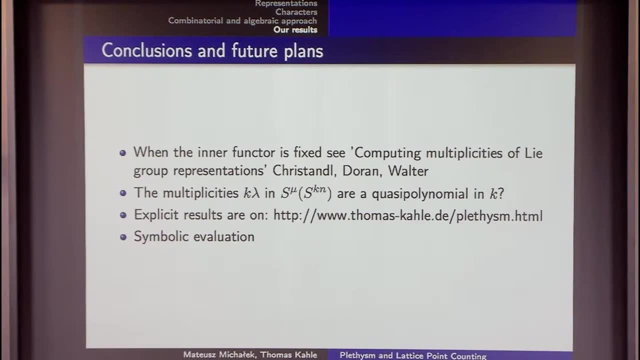 If you really want to see the formulas, I should say that these formulas, you can do much more than just asking for a multiplicity for a given K and lambda. You can evaluate it symbolically So, for example, you can test your conjecture. 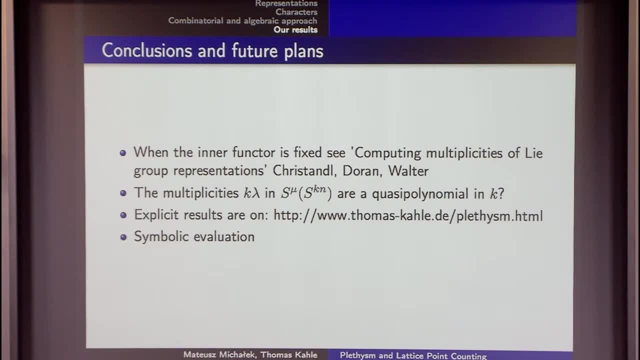 What's the multiplicity when the second row in your diagram equals the third one? So you just input lambda 2, equal to lambda 3, in our formulas and the computer does it for you. If you are lucky, the formula simplifies a lot and confirms or contradicts your conjecture. 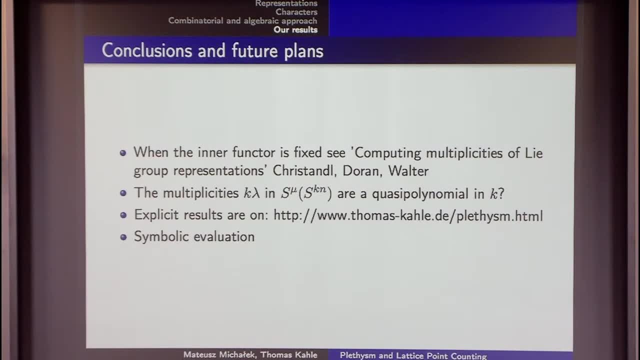 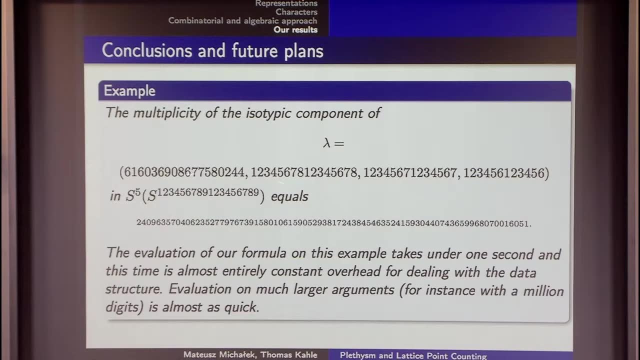 And then, how fast is the evaluation of an explicit formula? So here is an example. If you would like to know what's the multiplicity of such a random diagram inside such a plethysm, it's this And you are not supposed to see it, but the evaluation of such a formula, it takes under one second. 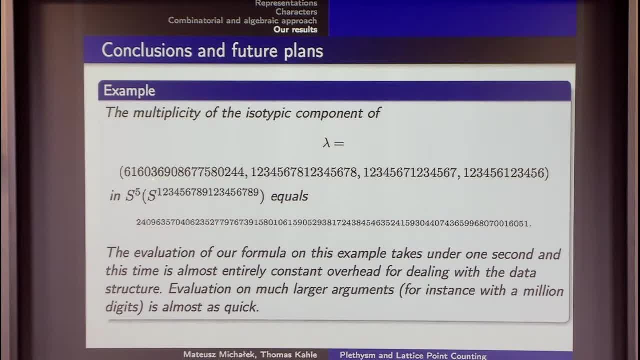 And Thomas said that we can do it when these numbers would have millions of digits. So explicit formula is like: really fast, There is no mathematics there, It's just showing that we can do it for really arbitrary numbers. Evaluate the formula, But up to S5 and even beyond. 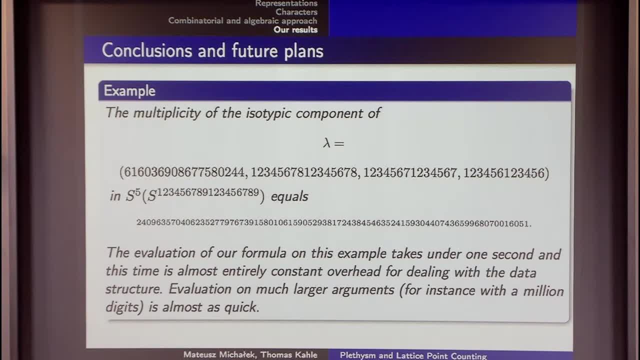 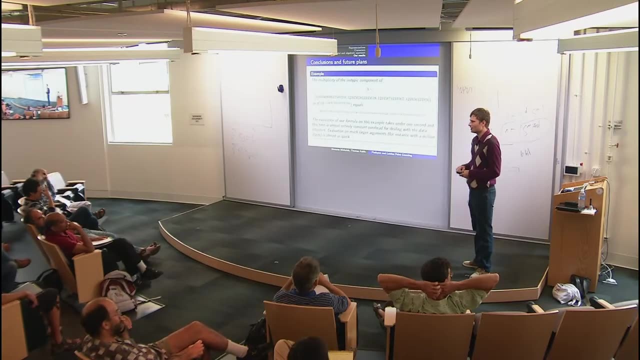 So we've got formulas up to S5.. If you would be interested in S6, we can probably push it. Well, there are a few tricks. We reduce the number of variables. We use the bar VNOC. Even such things as an ordering of summation play a big role in the computation. 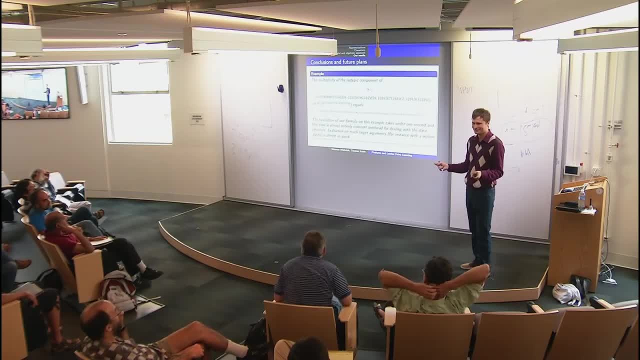 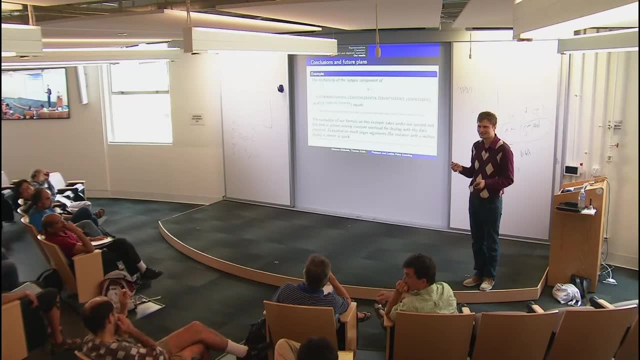 So we have sums And of course they are commutative. But choosing the right order in the summation, somehow the result depended on that. I cannot compute. There is a big FCM between the parts of lambda. 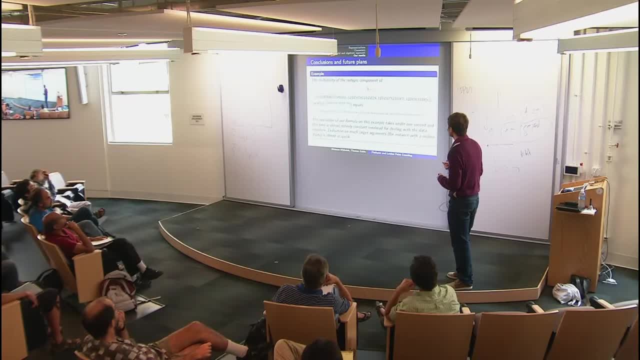 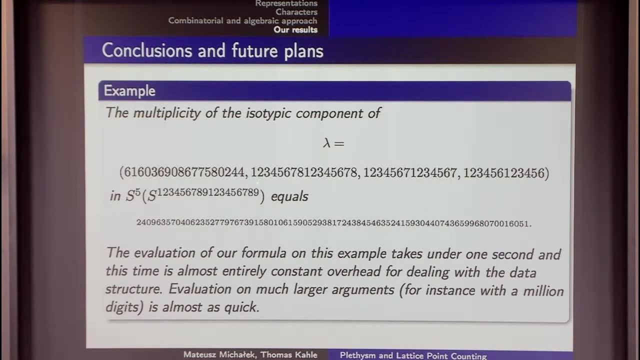 Sorry, A big gap, FCM. The parts of lambda Is lambda a multiple of some small. The numbers were random: 1, 2, 3, 4, 5, 6, 7, 8.. 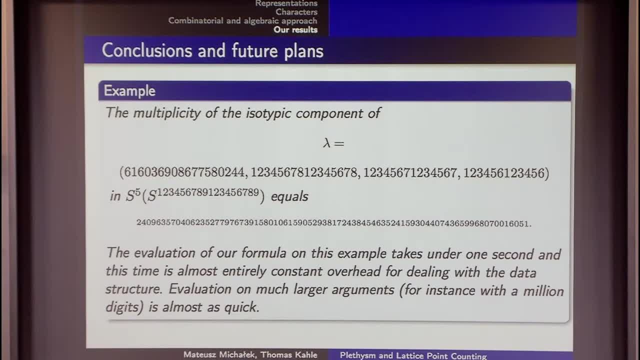 1,, 2,, 3,, 4,, 5,, 6,, 7, 8.. 1,, 2,, 3,, 4,, 5,, 6, 7.. It's random in binary representation. 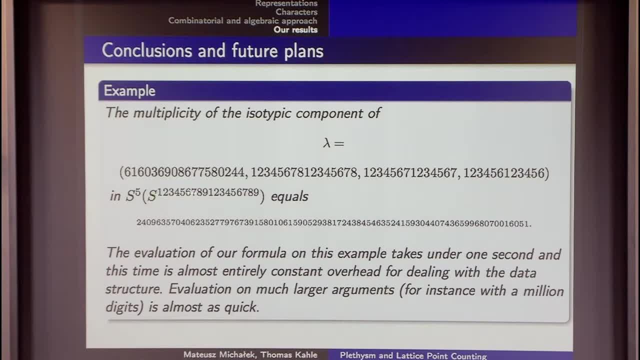 And the first one. what's that one? The first one is so that it makes sense. I mean the total weight has to be equal to 5 times 1,, 2,, 3,, 4,, 5,, 6,, 7,, 8,, 9.. 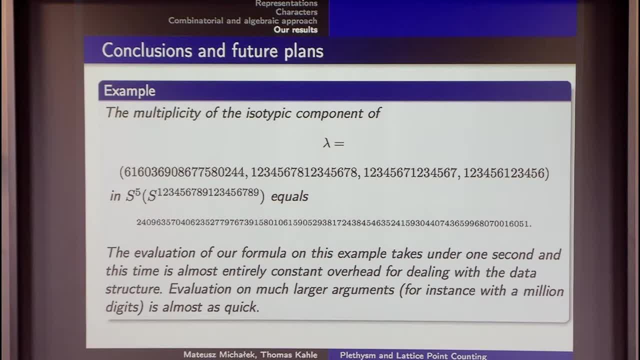 1,, 2,, 3,, 4,, 5,, 6,, 7,, 8,, 9.. Because otherwise it's 0. That wouldn't be interesting. Yes, that one. So I planned also to tell you what are the weak points of our algorithm. 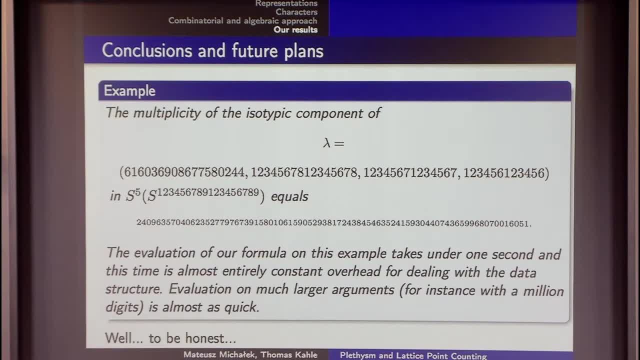 But I guess I don't have time, I don't have time, I have time. I can tell you. So there are a few very weak points of our algorithm. So this computer expert. So first of all, why this ISL library works so well. 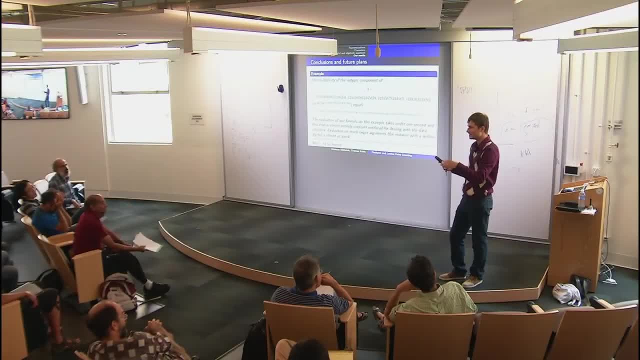 Because when you have loops in your program, four loops- this is like a parametrization of some geometric object in a high-dimensional space And they want to optimize four loops very well. So they want to have a better parametrization of this object. 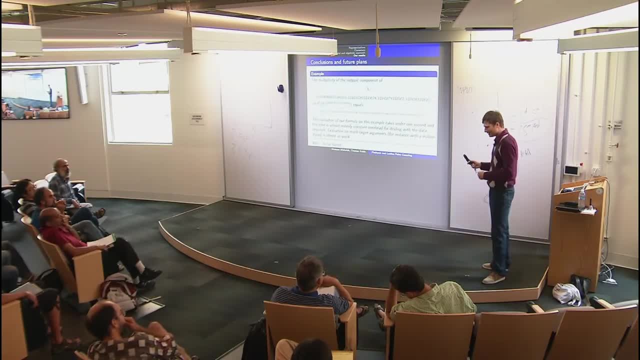 So they really work. So it's very hard to make these algorithms nice. But the things with algorithms and parametrizations inside them is that these formulas were never meant to be seen by human beings. But they've got the thing that transforms the computer formula into a human-readable output. 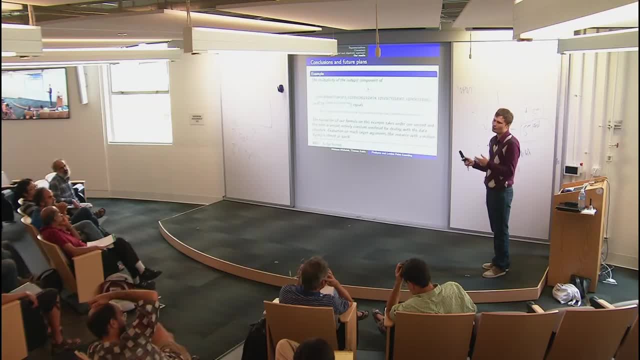 and read it back in, But it's very, very bad. They are working now on it and they are not very much interested. So our formulas are in human-readable output. But when you feed the computer, our formula into it. So our formulas are in human-readable output. 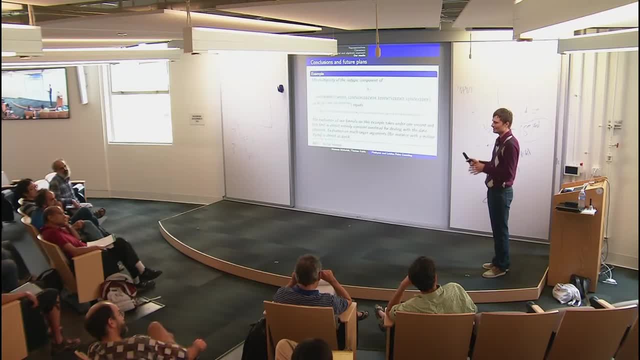 But when you feed the computer our formula into it, because this reading function is so bad, this takes time Just to read the formula. I mean it's not a huge formula, It's a few pages, So you can look at it being a human being. 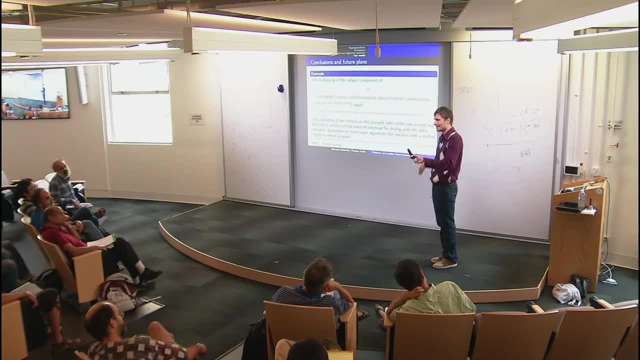 And once it's read in your memory, computer can edit, subtract it, do anything with it, like in fractions of a second. But they just didn't pay attention into the reading thing. So if you just want to do one evaluation it may take long. 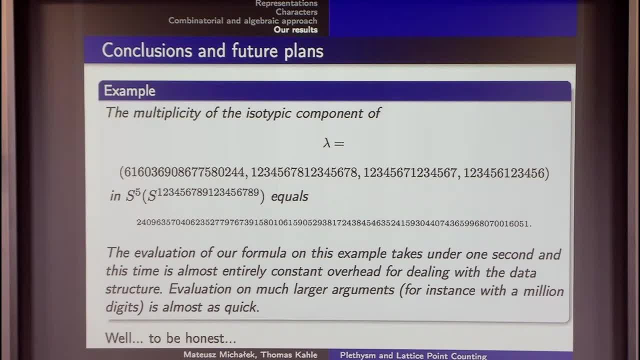 Because reading in our formula takes long. And another thing is we already know that our formula is a formula. It's not the formula. And the problem is that a function, for example, constantly equal to 2, you can present it as a function that is 2 for x, greater or equal to 0. 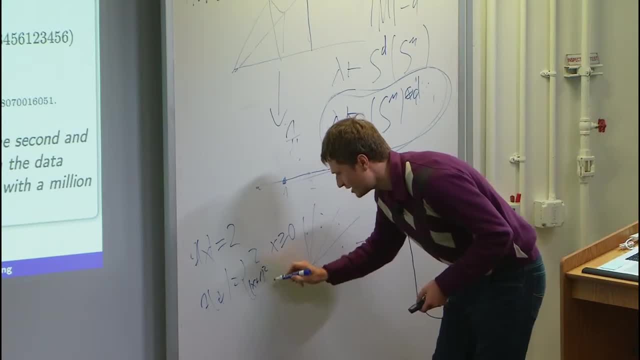 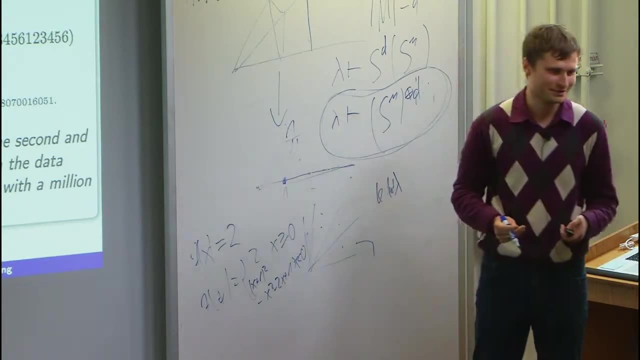 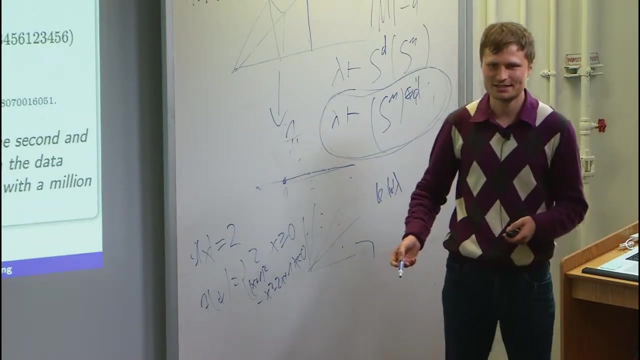 and x plus 1, square minus x, square minus 2x plus 1 for x less than 0.. I mean, you can do it, And the problem is that the computer cannot always join and say, oh, this is the same as this.